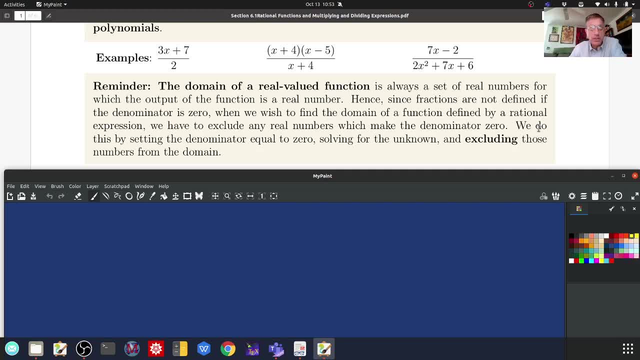 the largest set of real numbers, such that the output when plugged into the input- so x is the input- the output is f of x, such that the output f of x is also a real number. So with fractions we have always the problem. 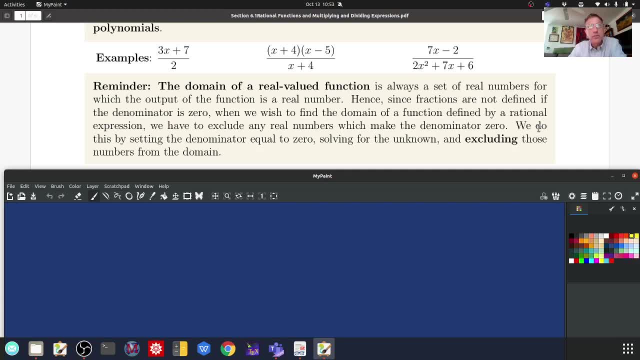 We can't divide by zero. So if inputting some real number into a function would result in division by zero, then we have to exclude that real number- or in some cases numbers- from the domain. So look right here at this example. 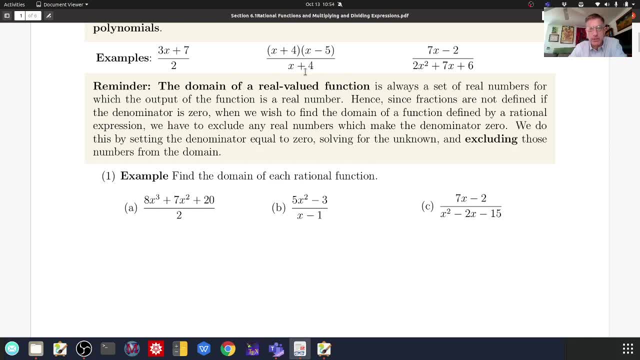 So this is a rational expression and we're just going to pretend it's a function, Like we'll actually do this right down here. So normally I would have f of x equals, and I don't know if it's just my laziness. on example one: 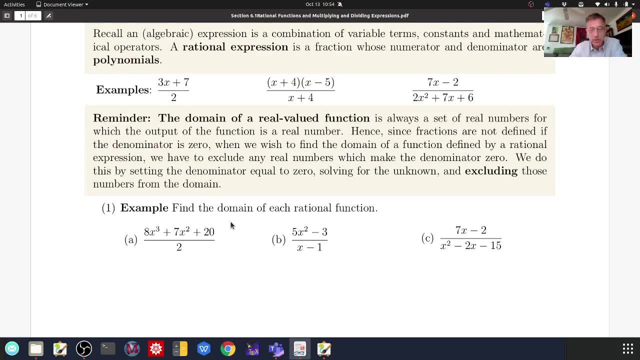 where the book just says: just pretend these are functions, But just suppose this is f of x. So in this case, if x were equal to minus four, then minus four plus four is zero and we would have to exclude minus four from the domain. 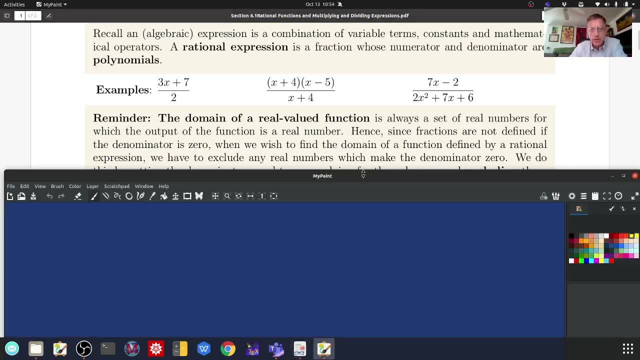 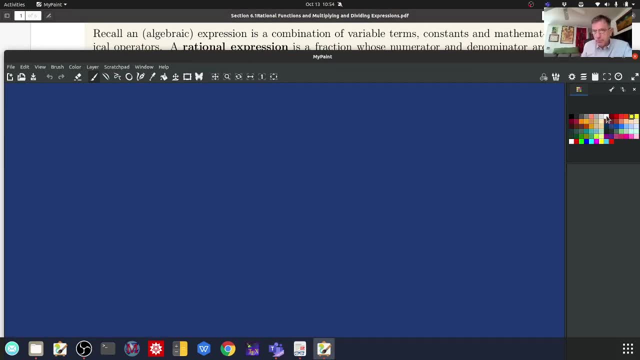 because we can't divide by zero. So let me give you an important fact. So this is just going to be a fact you can use In sight without justification. So we're talking about the domain, And domains are used in the context of relations or functions. 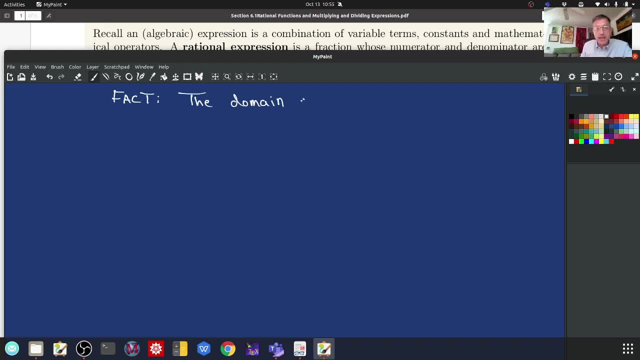 In this case, we're going to be talking about functions, The domain of any, And here's the keyword polynomial function. Ah, I spelled it right: Function is the entire real line minus infinity to infinity, But that only applies to polynomial functions. 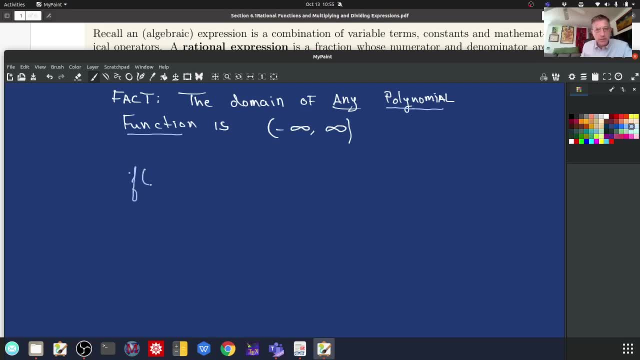 So remember a rational function such as f of x is equal to two x squared minus seven over five x minus three. The numerator is a polynomial and the denominator is a polynomial, We don't care. so that means their individual domains are both infinity to infinity. 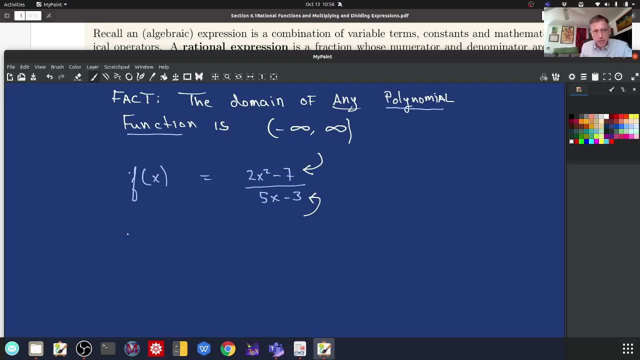 The real line, But we don't care about what their individual domains are, because we have created a new function by taking the ratio of one polynomial by another polynomial. So in this case we're talking about the domain of all of this right here. 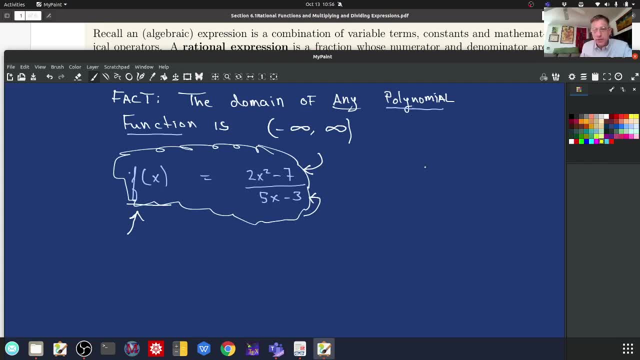 And what do we do to find it? We add a new function. We only care about the denominator, not the numerator. We want to find out where the denominator is equal to zero. So we set the denominator equal to zero And we solve for x. 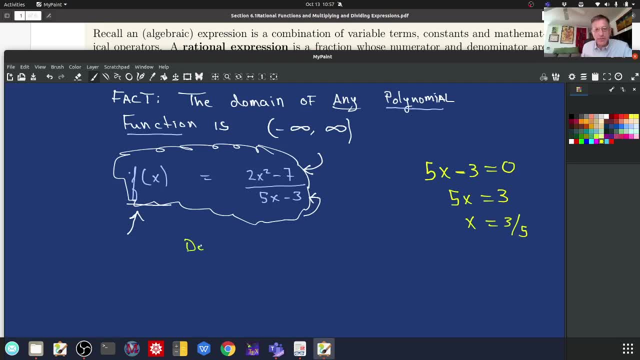 And then we write the domain. So the domain Of f is everything except three-fifths. So I start with minus infinity And I go all the way up to three-fifths by using the open symbol here for this interval. That means three-fifths is not included in the domain. 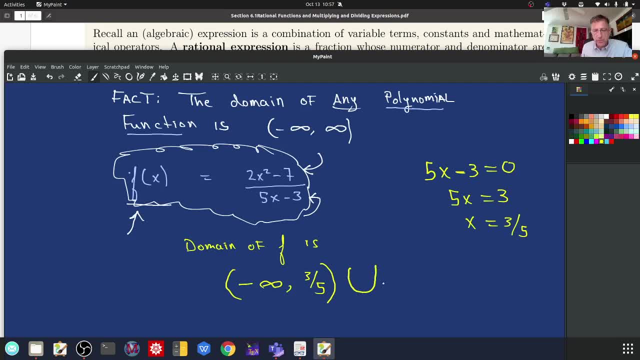 Then I take the union- Remember, the union looks like a? u- And I start again just on the other side of three-fifths And I go all the way to infinity. There are easier ways to write the set of real numbers. 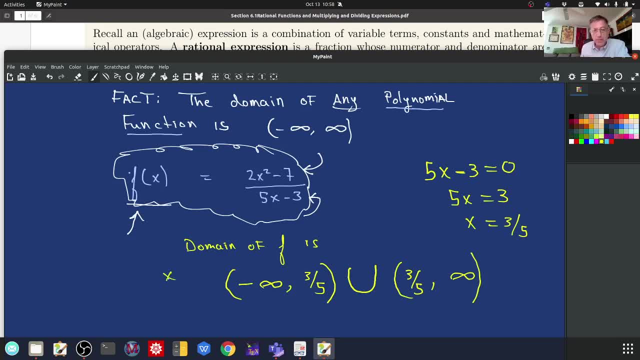 of all real numbers except three-fifths, But this is the way your book gives it. If you're curious, the real line is given by the symbol r, And if I want to write the real line I would just say r minus one element, three-fifths. 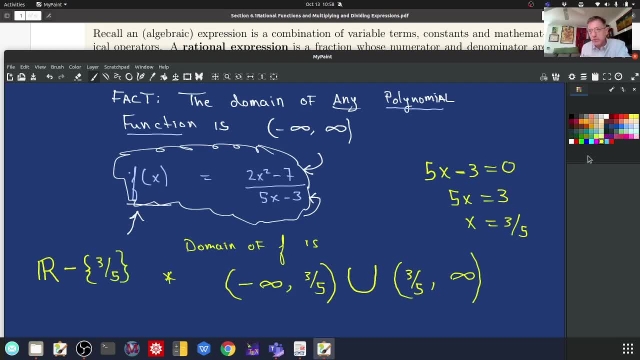 This kind of notation is beautiful set notation, But it's only FYI for your information. You cannot enter that in my math lab and get a correct answer. It won't understand it. This is what it understands And there's a reason we're focusing on introspection. 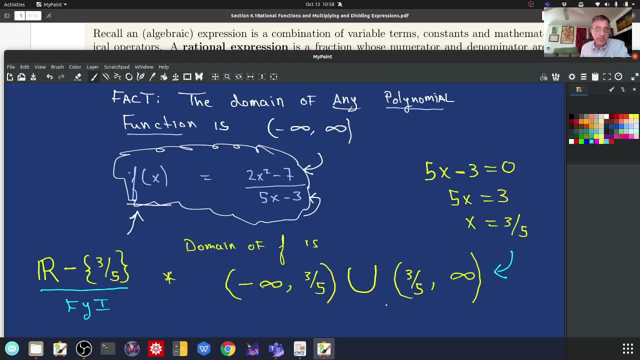 We're focusing on interval notation because many of the aim or the goal for some of you who are STEM majors will be to eventually get to calculus, And calculus is a subset of one of the great partitions of mathematics called analysis, And interval notation is all over in analysis. 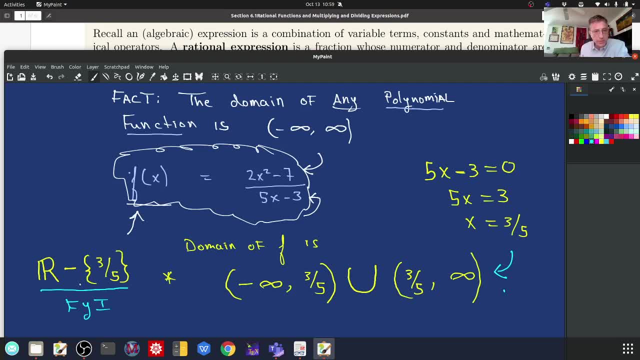 So it's good to use this. Of course, this is much easier to write. as far as set notation, It's just taking a few seconds Taking the real line and taking from the real line the one single element. three-fifths: 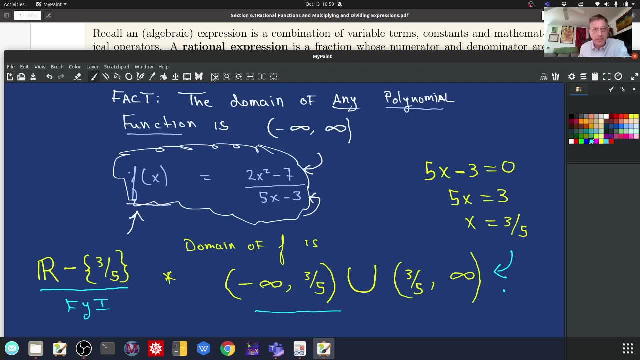 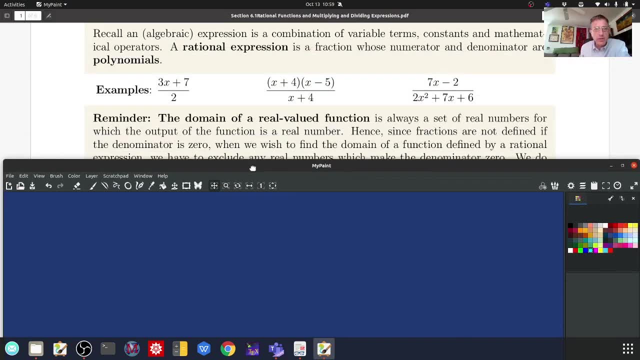 But this is what you have to use. A lot of you didn't care about that digression, But that's what the fast-forward button is for right, So let's actually do some. You've kind of already seen what we're going to be doing. 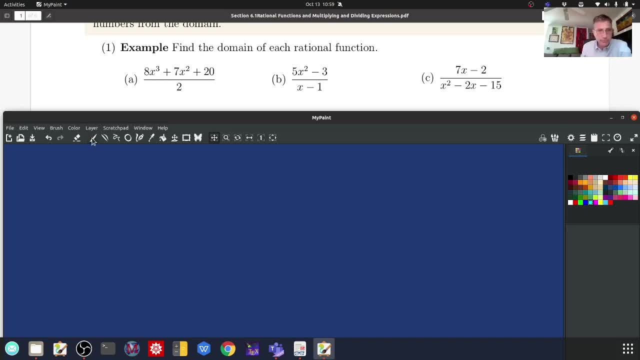 So we're going to find the domain of the following rational functions. So we're just we're going to- I don't want to pause the video and check the book. I'm pretty sure this is exactly how the book writes them. I usually try not to deviate it, but I just want to make sure you understand that this. 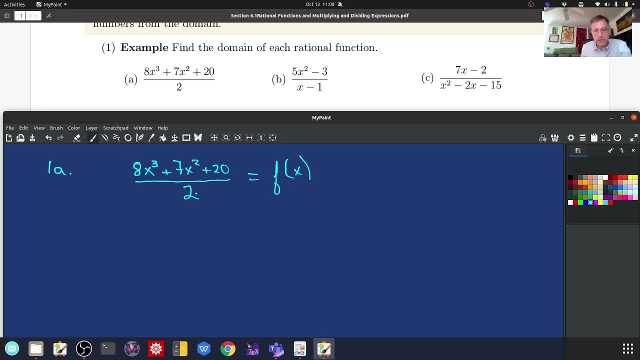 is a function. They say it's a function, so it's understood. So all we have to do is we can assume. Well, our assumption is: the domain is all real numbers minus. that means we're excluding them from the set- any real number or any real numbers, because many times there's going. 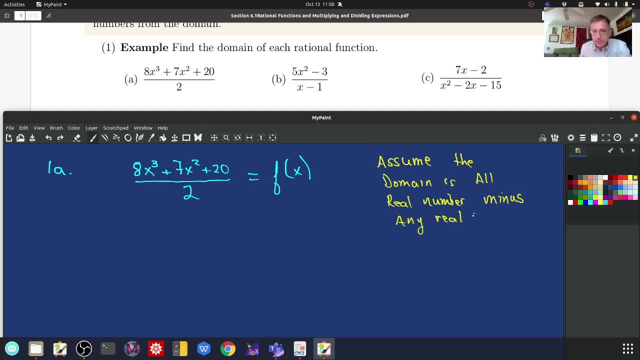 to be more than one- And you should be able to finish the sentence for me- that make the denominator zero. So there are no real numbers that make the denominator zero, Because the denominator is a constant. So the domain of 1a is minus infinity to infinity. 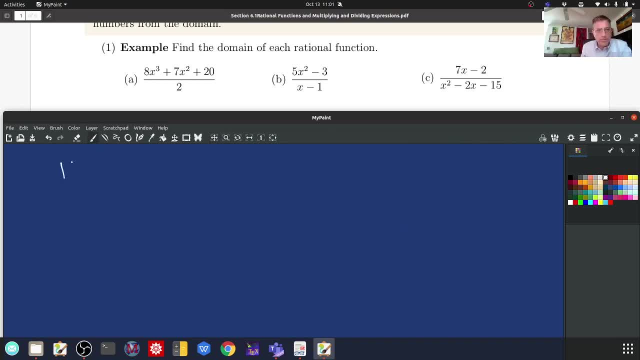 So for 1b we'll have f of x equals 5x squared minus 3, over f of x squared minus 3 over f of x minus 1.. We don't care about the numerator. All we do is take out the denominator and set it equal to zero. 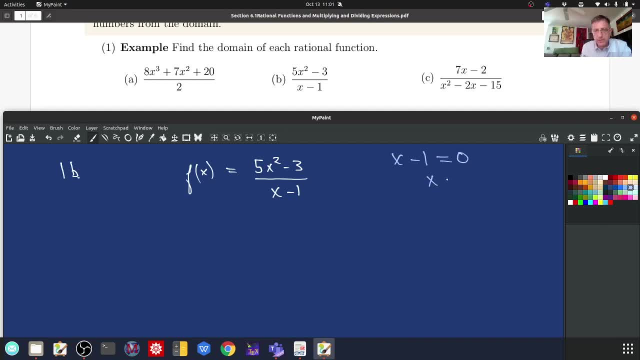 And I write the domain and the domain of 1a are all real numbers except x, And this is how they want it. seen in my math lab, I am assuming Some times this rule doesn't apply to everything, So now we'll try to accumulate it. 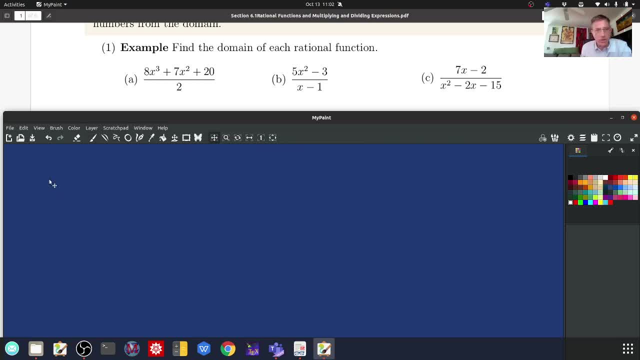 This is just the 15エ, and now we're going to subtract everything out of process. they can surprise me at how they want things written, And this is 1C. 1C is a good example. Let me readjust here. I've been writing so much my fingers are really sore from writing. 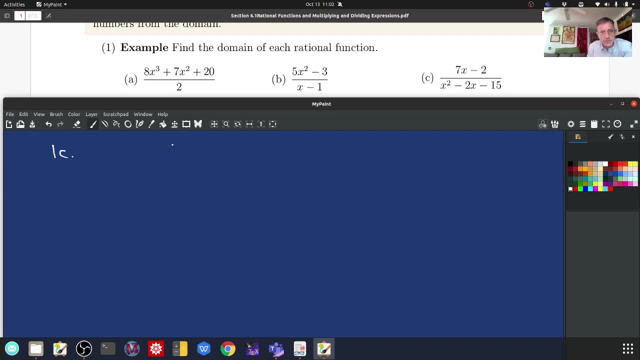 So if my writing looks really odd, it's because I've been. this has been a week of exams for me and I just don't like to give exams and grade them, unless you get some kind of comments. So anytime you miss something, if I can read your writing and find out what it was you 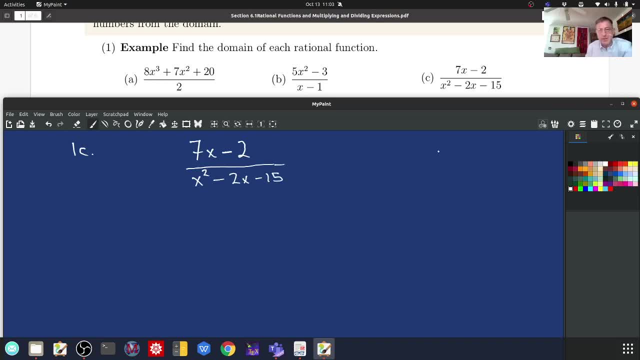 get a comment. That's a lot of typing. I've just discovered an app in Chrome that allows me to speak what I want to say, and I'm using that because my fingers are shot. So, in this case, what we have to do? 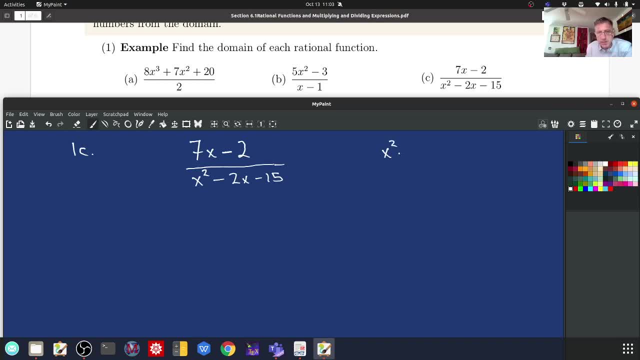 is. again, we look at the denominator and set it equal to zero. So what do we do? We have to factor. The only way I can solve this equation right here is to factor, And you will always be able to factor it. So, factoring the GCF of X squared. 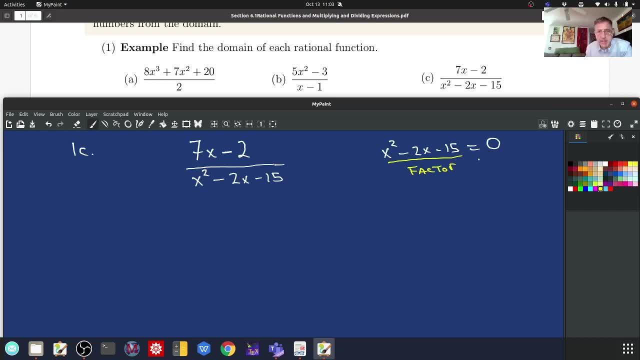 minus 2X N minus 15 is 1. So I can't remember бол sharing all your written � rainy days. I can't remember бол factor out anything so we'll go ahead and factor this really fast using the tic-tac-toe method or whatever you want to call it I noticed a lot of you using 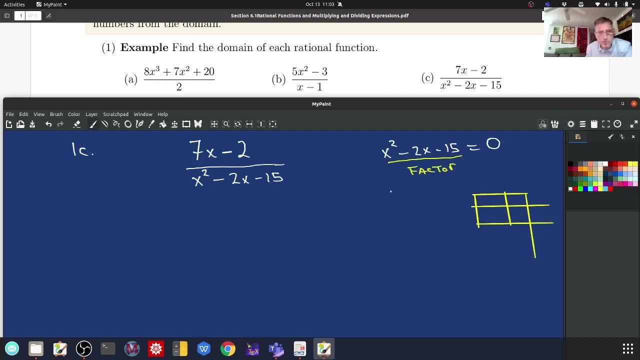 it on the exams that I'm still in the process of grading, so I need x squared here, minus 15, and my middle term is always the bottom term, since it's monic. that makes it easier. that's X and that's X. now, 15 is 5 times 3, but one of 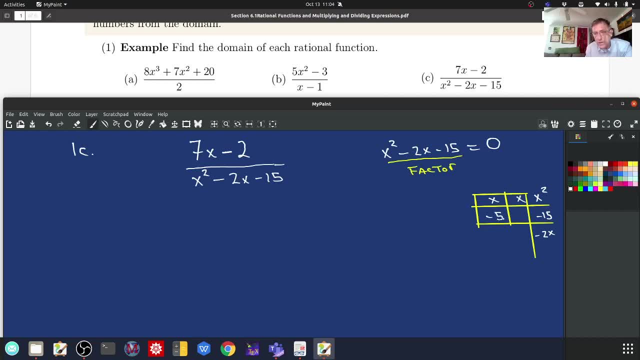 those have to be negative and we want to be the larger of the two to be negative, since when I add them I have to get minus 2x. so this gives me my factorization. so the factorization is X plus 3 times X minus 5 is equal to 0. that's the reason factorization is. 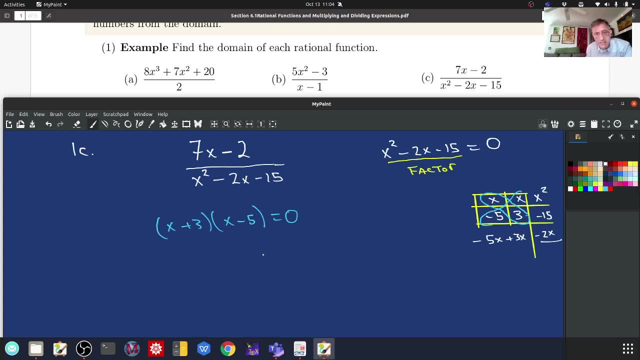 really important for the rest of this class, and then I just set each individual factor equal to 0. this is basically something we've already done and you've actually just been tested on it. the test questions are pretty basic because you're going to have plenty of opportunity. 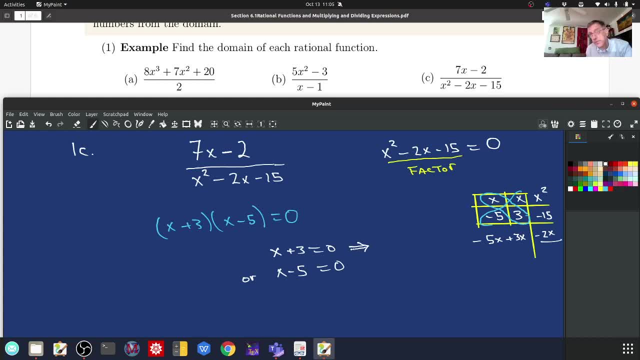 to factor harder polynomials in the in this chapter 6 text test. so this gives me X is equal to minus 3 and this gives me X is equal to 5. so how do we write that in the interval notation? this is where you just have to get the pattern. so if you 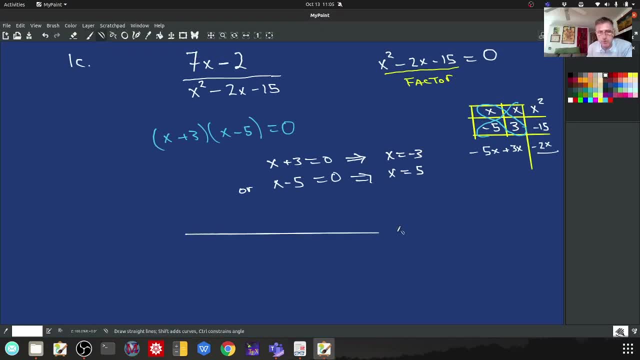 want. I actually show you this on the number line first, just one visual, and that may help. so here's my number line, the number line. when I say the real line, that's what I mean. the real line is just the number line and you can put a zero. 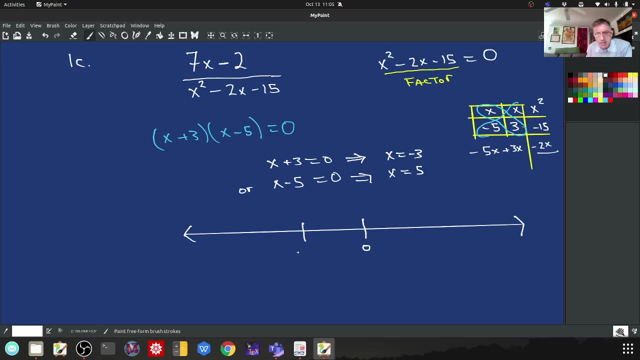 there if you want. now I'm going to say minus 3 is here, but we don't want minus three in my set. I'm going to say five is right here and we don't want want it in the set. So I start at minus infinity and I go all the way up to minus 3, but I don't. 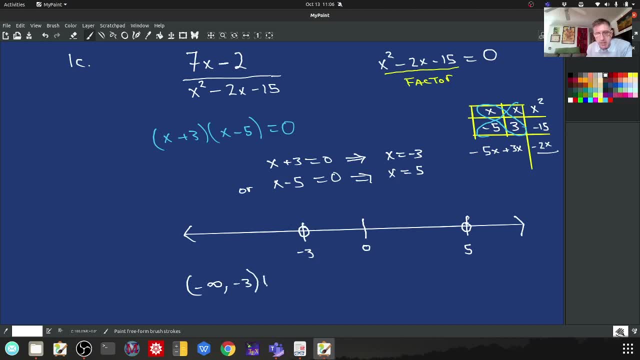 include minus 3.. Then I take the union of another set and then I start at minus 3, but don't include it and go all the way to 5.. But I don't include 5 either. Then I skip over 5, and I start at 5 and go. 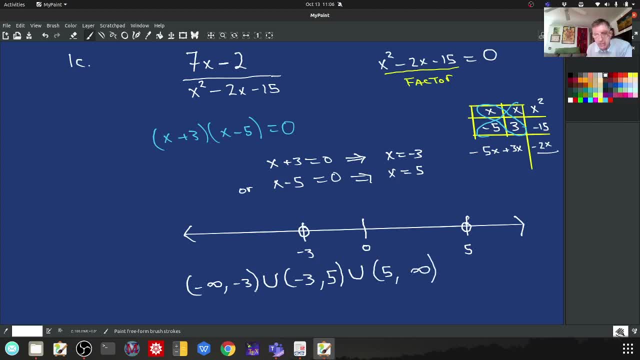 all the way to infinity, but in each case I don't include them. So all of this is an open interval. This is the union of three open intervals. This interval is called an open interval because I'm using these types Of parenthetical- I guess- braces, I don't know- brackets, And this is closed And this is half open. 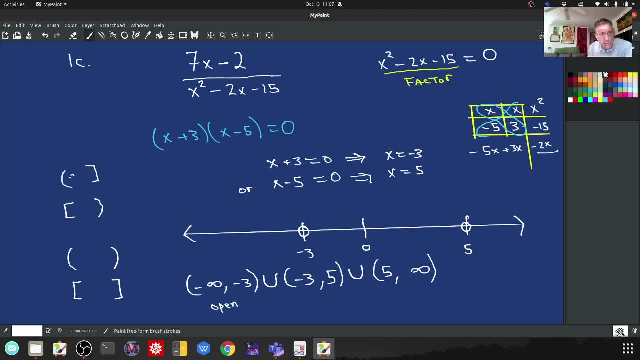 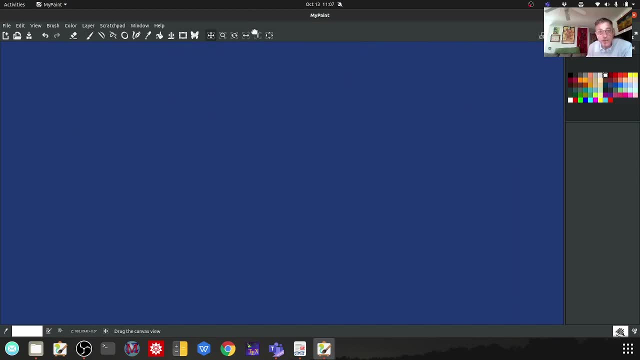 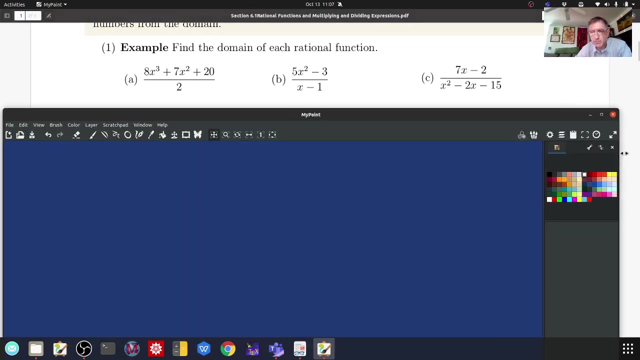 half closed, half open, half closed. So just a reminder there. Okay, so not so bad right. I'm hoping you feel pretty comfortable with this part Now, if I can just make this get smaller. Okay, mouse time. Let's look at the next problem. Oh, we did all those problems, So now we're going to 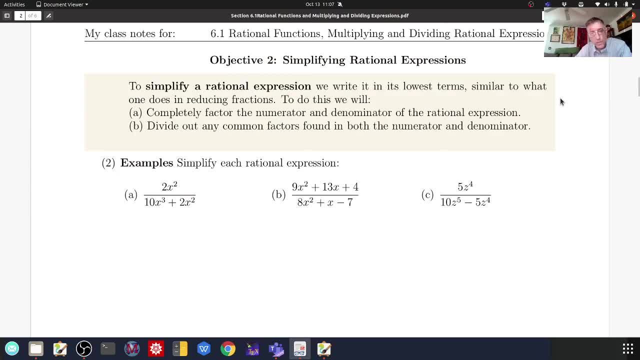 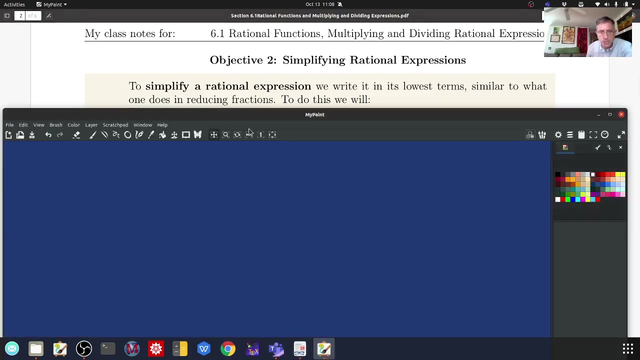 simplify rational expressions. So what does it mean to simplify a rational expression? Just like when you simplify a fraction, you reduce it to its lowest terms. That means factors that are in the numerator and in the denominator cancel out. It's exactly what we were doing when we would simplify. 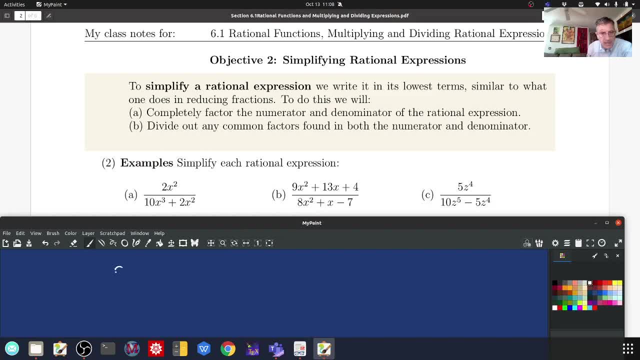 something like a to the sixth, power over a to the fourth. Well, I have six factors of a in the numerator, four factors of a in the denominator, so they cancel out, I get to cancel out four. There we go, So what I have. I have two factors of a in the numerator, a times a, And remember which A's get. 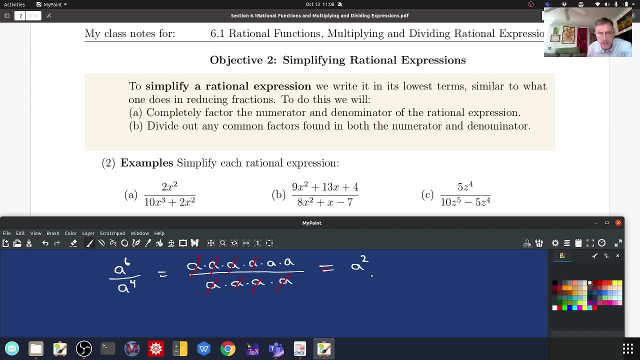 canceled out first. So a gets canceled out before A gets canceled out before four. That makes is the right number, Number Number. Remember ammunition, How it gets canceled out first. So the difference from A to A it's going to depend onнюr. OK, I'm somewhat afraid I make that one too person. Bigoke didn't see that. call just there. Take notice of the hexagons. OK, So you can notice the grid. you take note if there is, of course he's going to get screenshot. 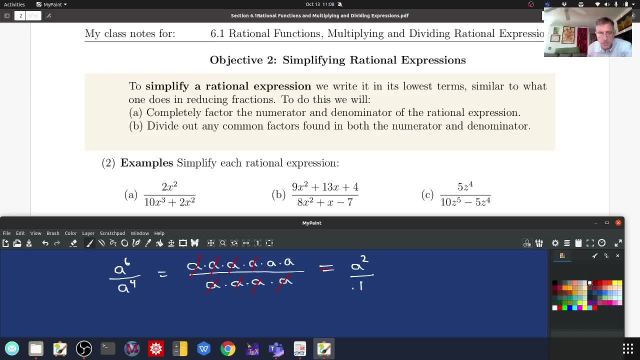 Look at this oneeltron spML que if you are ever going to see that color. when you cancel out, they don't become zeros, they become 1.. So it's a squared over 1, or just a squared. Well, the same type of procedure is going to be working when we simplify each rational. 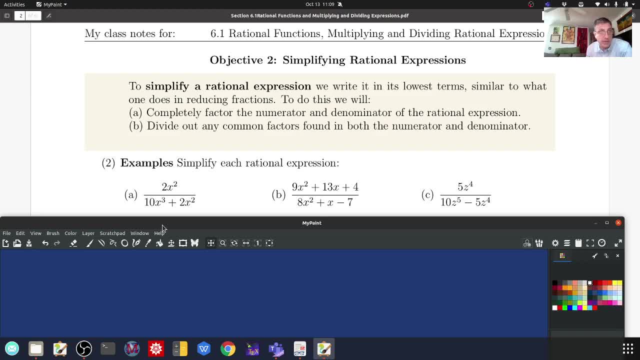 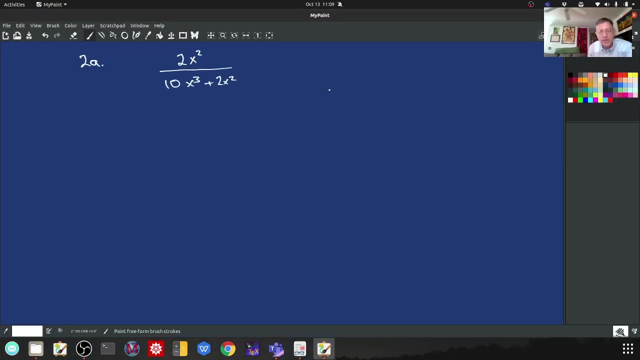 expression. We completely factor the numerator and the denominator and then cancel out like expressions. So here's my 2a, So I have 2x squared. It has a really easy numerator And then I am dividing over 10x cubed plus 2x squared. So what we do is we simplify. 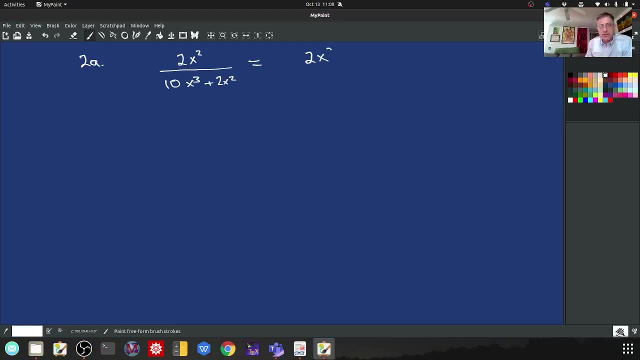 The numerator cannot be further simplified, so I'm just going to copy it over. Let me turn my page here. Yeah, I just want to make sure I've copied this down right Now. for the bottom we have to factor out the GCF. So the GCF of these two terms- well, the GCF of 10 and 2 is 2,. 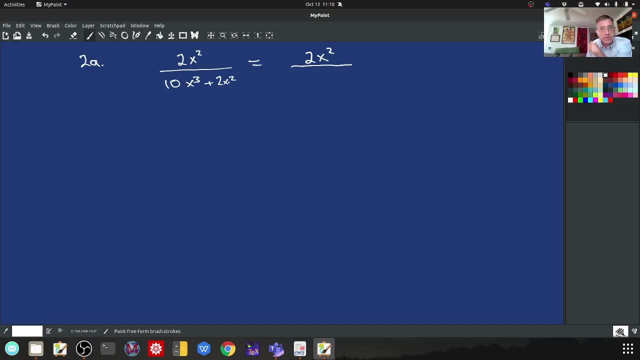 and the GCF of x cubed and x squared is x squared, So the GCF is 2x squared, So that's the GCF and I'm factoring it out. So 10x cubed divided by my GCF is 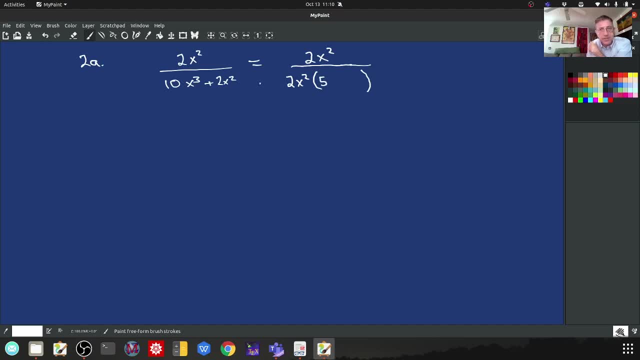 well, 10 divided by 2 is 5, and x cubed divided by x squared is x. And then plus 2x squared, divided by plus 2x squared is plus 1.. So it's been simplified as far as the factorization element. 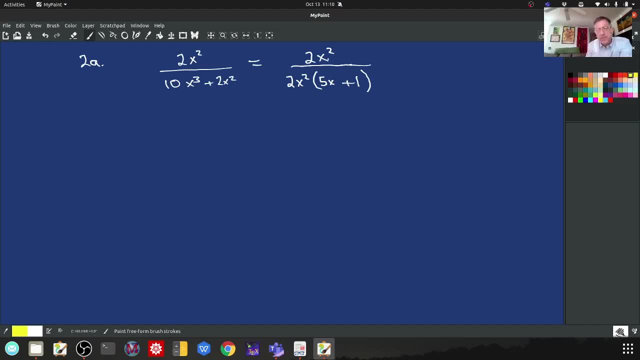 goes as much as I can, But if we look, 2x squared is the same in the top as in the bottom. So what do I get? They cancel out. Remember, when you cancel them, they become 1.. So the numerator becomes 1,. 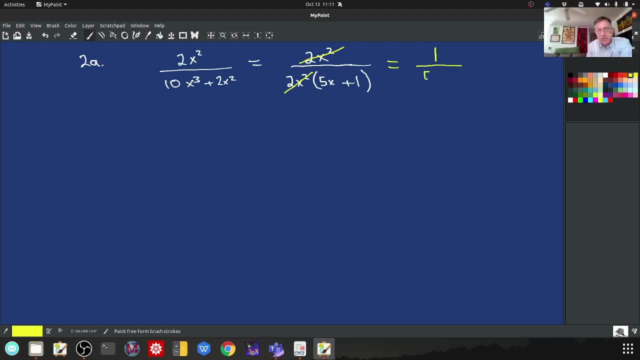 and this is 1 times 5x plus 1, which is just 5x plus 1.. So just a reminder: these are products 2 times x squared, And then I have that exact same product down below 2 times x squared. 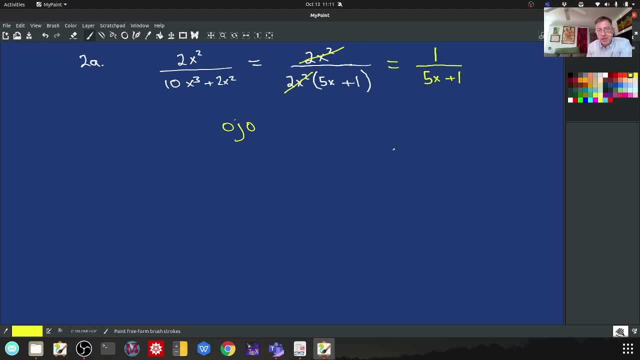 Now what can be factored out? If I have 5x plus 3 and 5x minus 1, this is wrong and it's a common error. You cannot cancel out the 5x's, because these are is the sum of two terms and the difference can't do that. 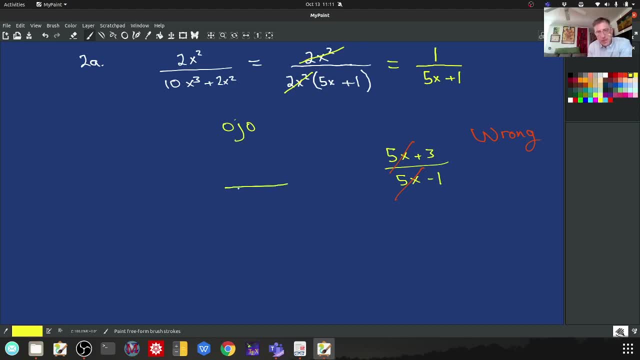 What could you do? Let's try this: If I have 5x plus 3 in the numerator and 5x plus 3 in the denominator, then these represent the exact same value or quantity. So those could be canceled out and I would get 1.. 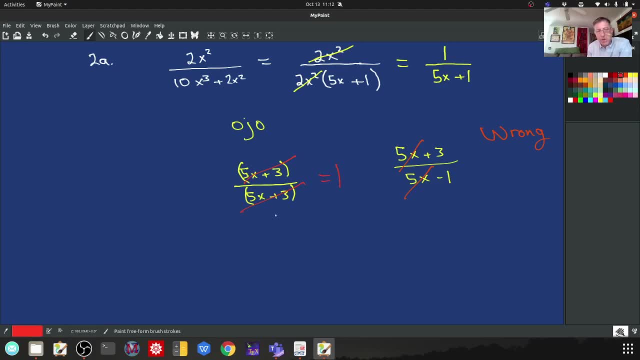 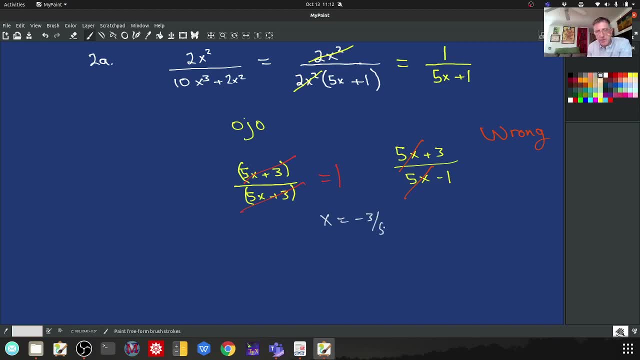 1. 1. 1. 1.. x is not equal to minus three-fifths, because if x were equal to minus three-fifths, the whole expression is undefined at that value. So let's go ahead and do another one. 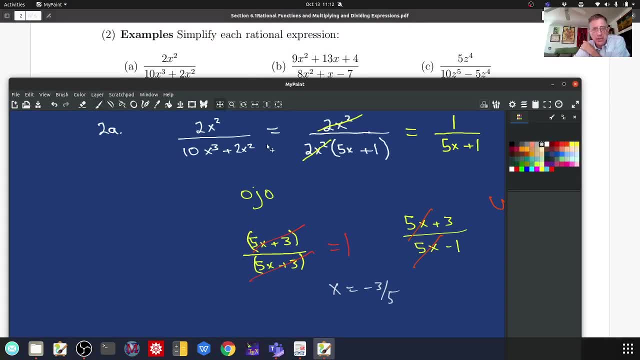 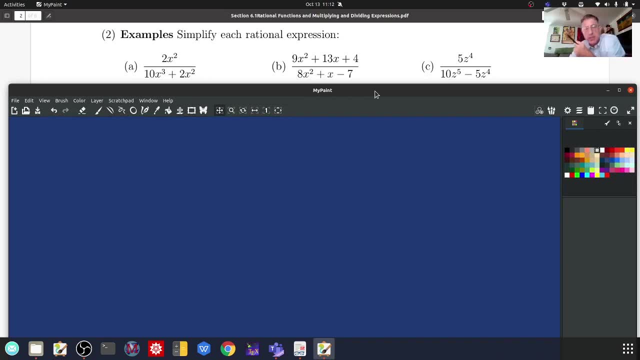 See, there's going to be a lot of factorizations here, so you have to get really good at factorization, And sometimes you're going to be factoring polynomials, and sometimes you're going to be factoring binomials, And to factor a binomial you literally just look for the GCF. 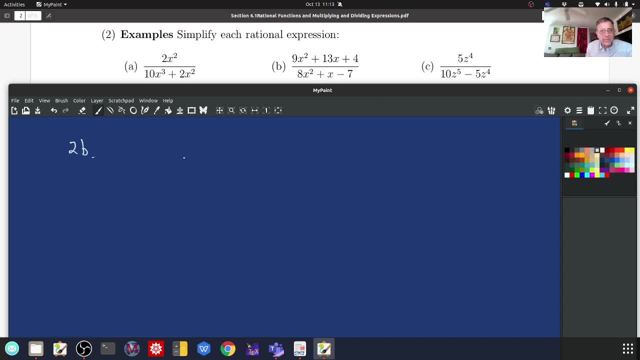 So let's do 2b, So 9x squared. Now I'm not going to do that. If I factor all of these for you, it will take forever to get through this lecture. so I'm not In each case, I'm just going to factor one of them on paper for you. 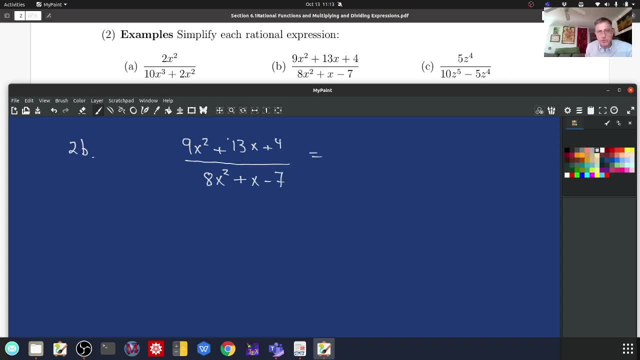 or in the lecture, and then I'll let you verify or factor on your own the other. So here we have two polynomials, And I'm going to go ahead and I'm going to just simply declare that the factorization of 8x squared plus x minus 7. 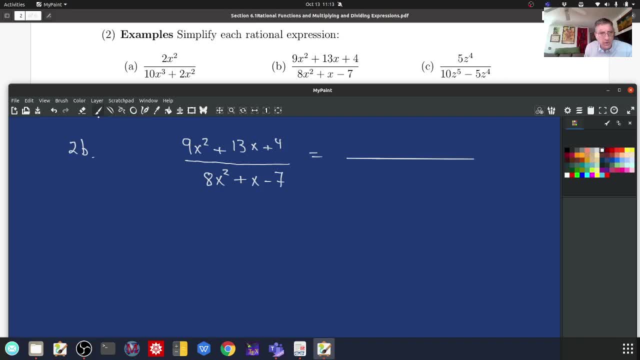 is 8x minus 7 times x plus 1.. And you can quickly verify that. Just spoil it: 8x times x is 8x. 8x squared minus 7 times 1 is minus 7.. Minus 7x plus 8x is x. 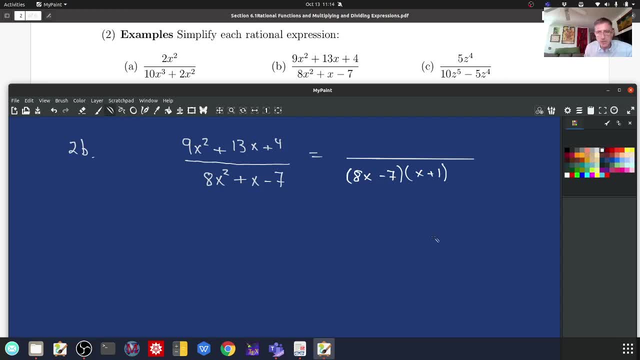 So let's go ahead and factor using the known method. Some of you- it looked to me like on the exam- have another method or you've already simplified the method I've given you. Like I said, this method, you can use any method you want. 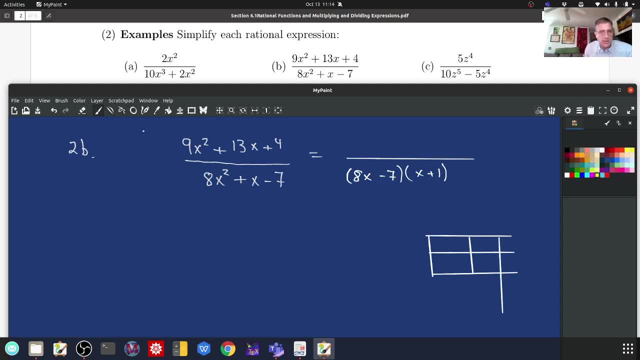 as long as you're able to clearly demonstrate that it's you who are doing the factoring. And so this is an interesting one, because 9x squared- the square root of 9x squared- is 3x, So the first term is a perfect square. 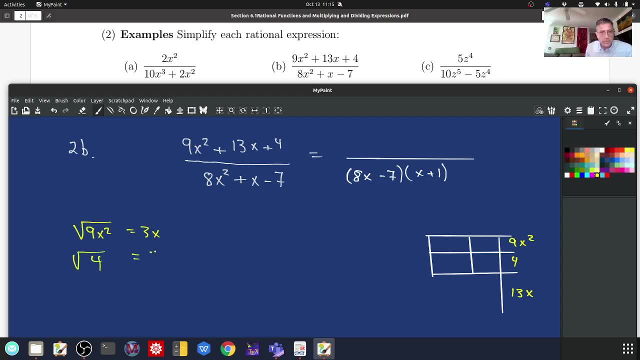 and the square root, So 4 is equal to 2.. So this is almost a candidate for a perfect square binomial. But if I multiply- remember we have this new factor, It's called the cross term factor- If I multiply 2 times what I'm given here, 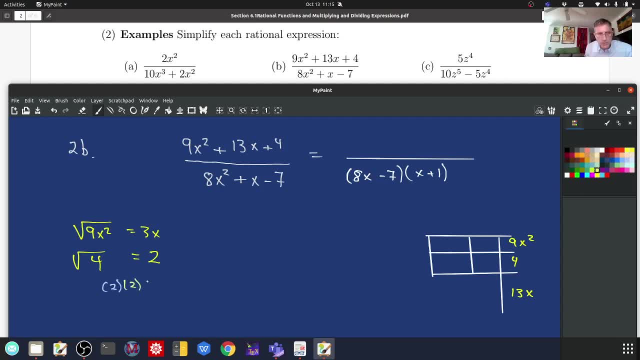 times 2 times 3x, I get 4 times 3x, which is equal to 12x. So if the middle term were 12x, this would have the factorization of 3x plus 2 squared, But my middle term isn't 12x, so I have to do it this way. 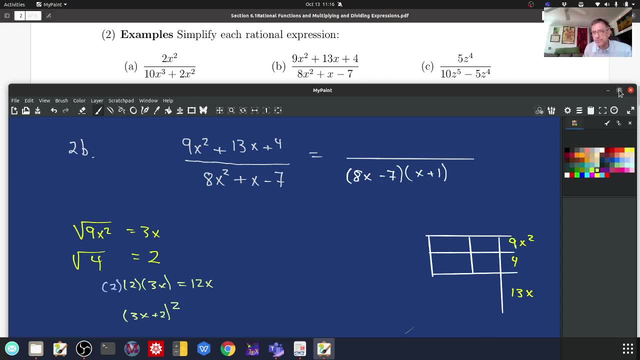 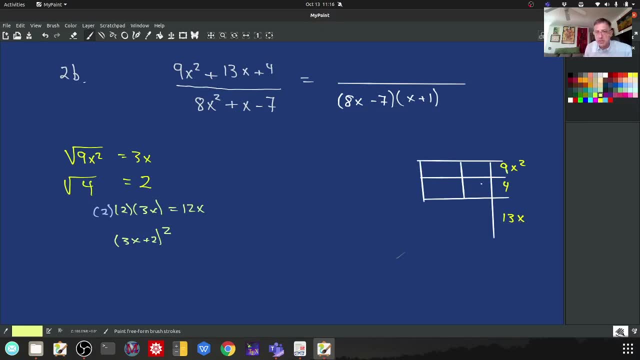 So a lot of choices here, and they have to add up to 13x. So let's do 1 and 4, 9x and x, Okay, so 9x times x is 9x. So 9x times x is 9x squared. 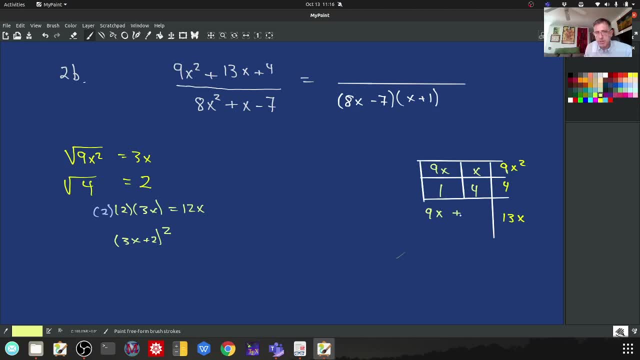 1 times 4 is 4.. So that's 9x plus 4x. So that gives me 13x. So my factorization is 9x plus 4.. Remember, we're going kitty-corner in x plus 1.. 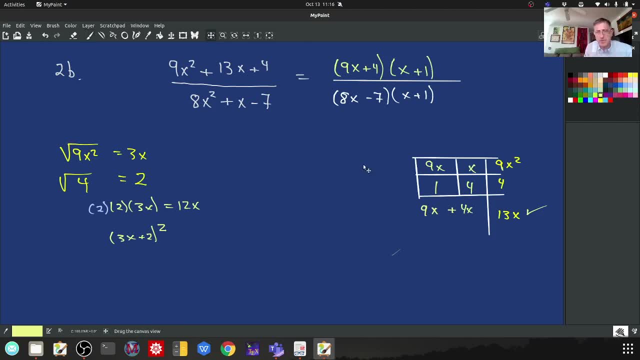 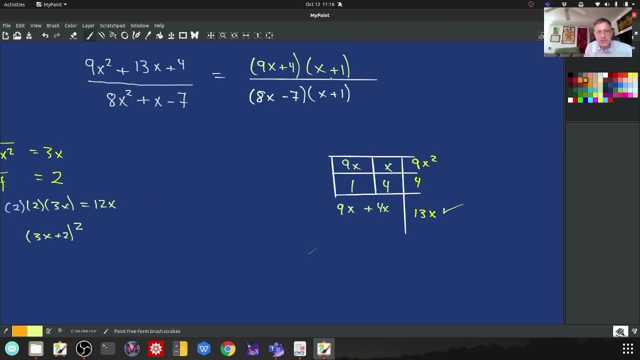 So now the numerator and the denominator have been factored And now we cancel out like factors. So the only like factor is x plus 7.. So the final answer is 9x plus 4.. It's okay if you keep it in parentheses. 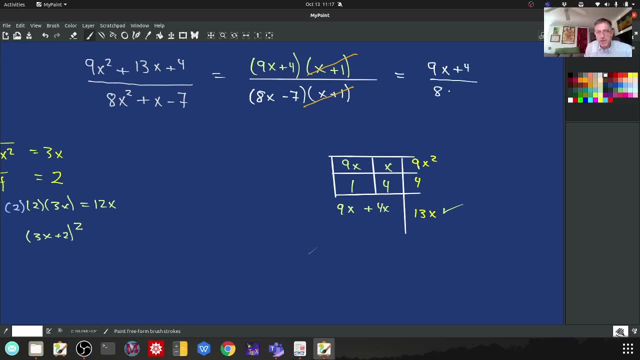 But there's no need to over 8x minus 7.. Just realize there's nothing you can do with that 9x and that 8x. This is it. This is done Why? Because 9x plus 4 is a prime linear factor. 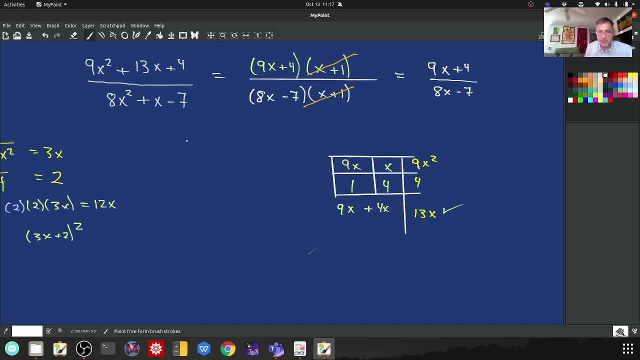 And 8x minus 7 is a prime linear factor, Just like if you had 7 fifths as a fraction. you can't reduce that. 7 is prime and 5 is prime. That's fully reduced, fully simplified. 9x plus 4 is a prime linear polynomial. 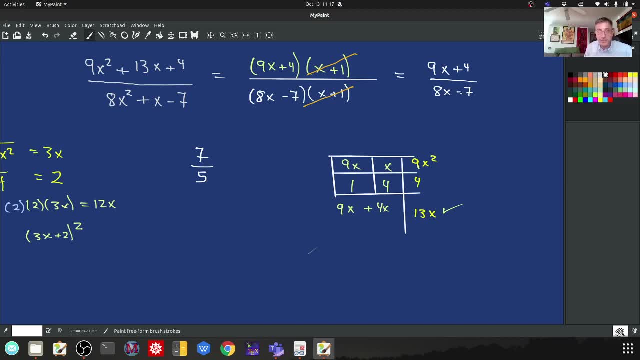 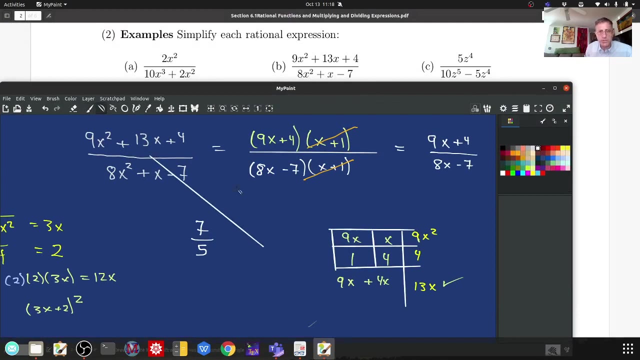 It's a binomial And 8x minus 7 is a prime binomial. By prime means there is no further factorization. So remember, the process of factorization is changing sums into products. Well, not that, Here we go. 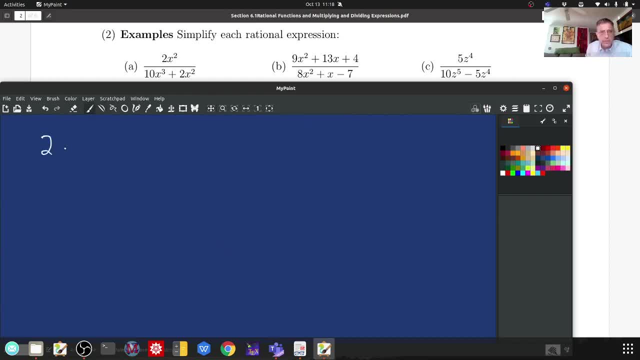 So let's do number 2c. So here this is not going to be bad. 5z to the 4th: There's nothing that can be done. That's a single term, So there's no factoring possible there. 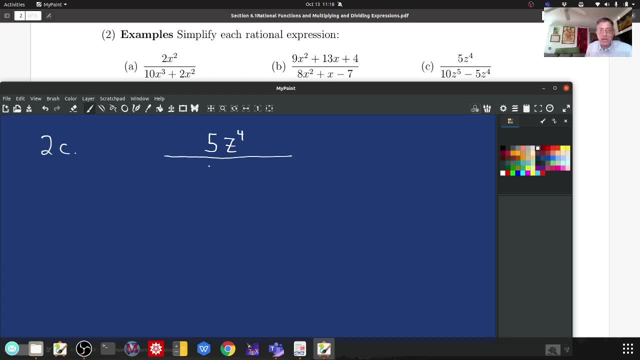 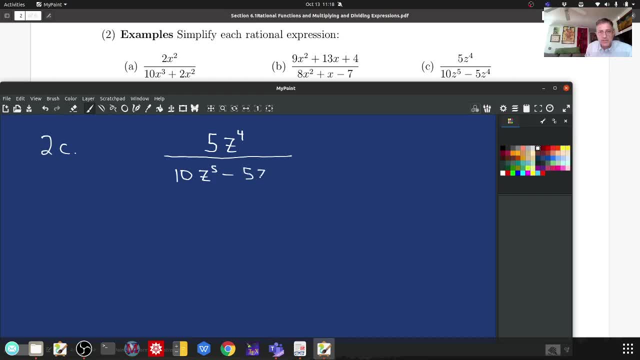 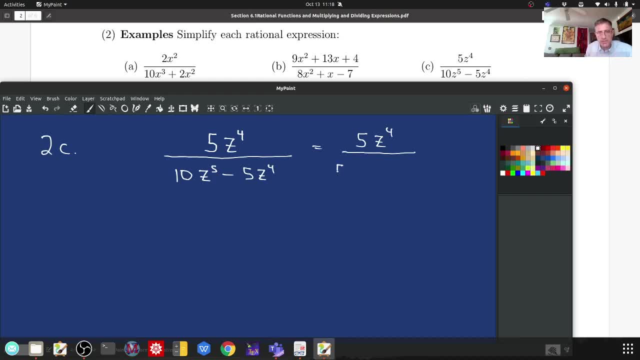 So the GCF of 10 and 5 is 5.. And the GCF of z to the 5th and z to the 4th is z to the 4th. So 10z to the 5th to the fifth, divided by five Z to the fourth is two Z minus five Z to the. 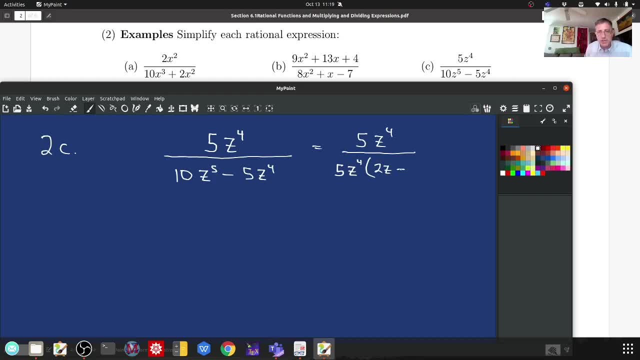 fourth divided by five Z to the fourth is minus one. and now, as you can see, we do have a common factor in the numerator- five Z to the fourth- and the same factor appears in the denominator. so again, this doesn't go to zero, it goes to one things. 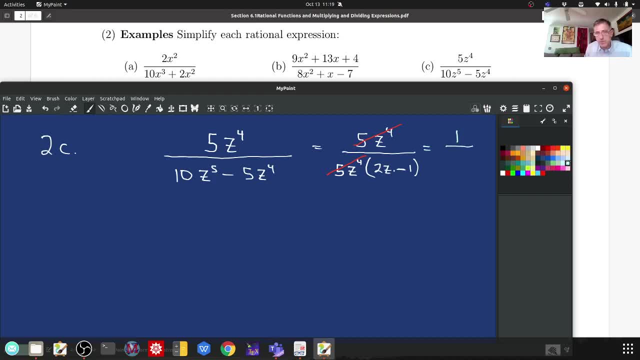 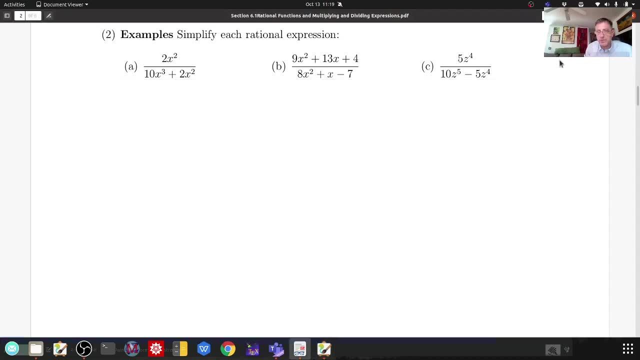 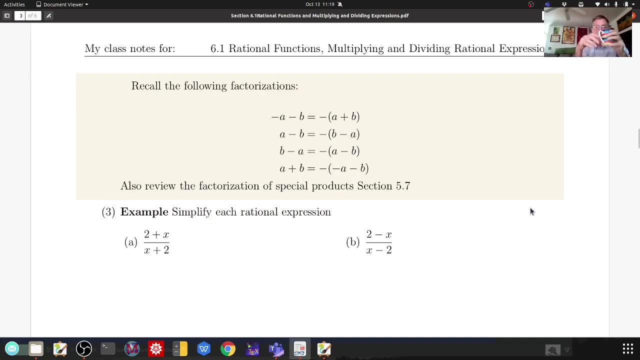 cancel out, turn into ones. this is one times two Z minus one, or just two Z minus one. so these are really important. this is something that should go in your notes. this is called Fibonacci- Fibonacci factoring out a negative one. so if I have minus a, minus B, I just factored out. 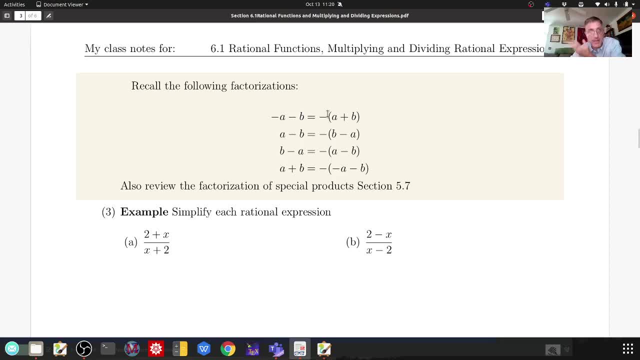 a minus one. I don't put minus one there, I'm lazy and I just put minus. so that's minus a plus B. a minus B is minus in parentheses. so notice what I'm doing. all I'm doing is I'm writing parentheses, I'm putting a minus in front of it and then 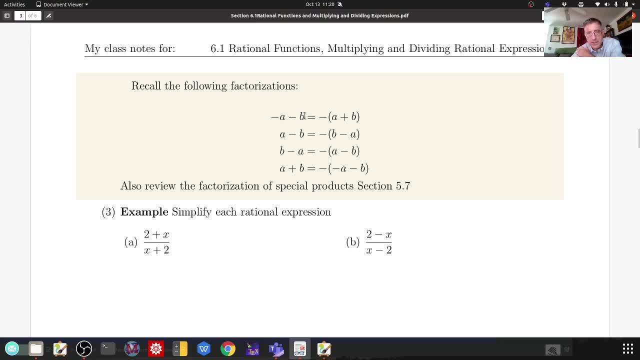 what goes in the parentheses is the opposite sign of what's existing. so the minus a becomes a positive a. so we don't write positive and the minus B becomes plus B. and we do write a plus B because we're. it denotes addition here. so these are things to keep in mind. we will be using. 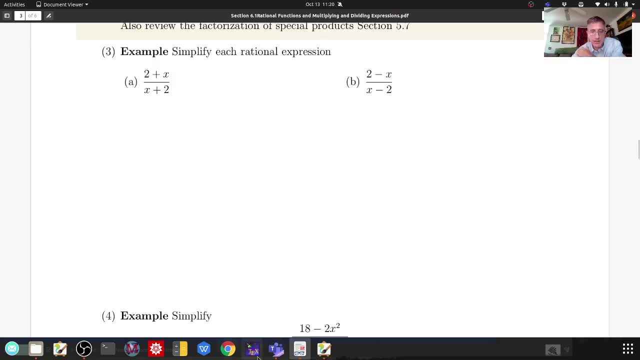 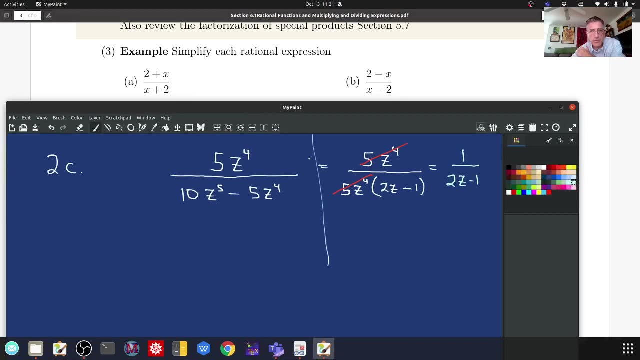 them. as a matter of fact, we're going to be using them right here in example three. it's a really important factorization tool. we're going to use all of our properties of real numbers to do all of this. so 2 plus X divided by X plus 2. but I'm now going to use the commutativity of a. 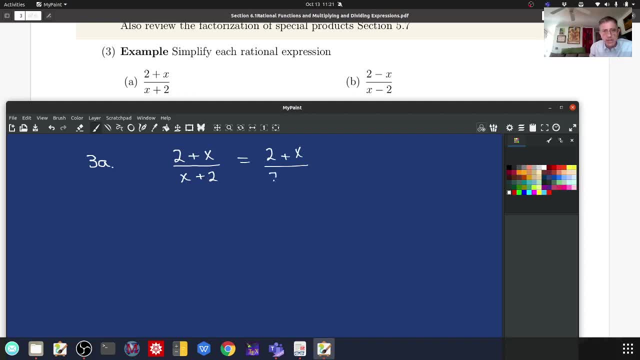 addition to write: X plus 2 is 2 plus X. now 2 plus X in the top is the exactly the same as the 2 plus X is the bottom. so that's equal to 1, provided X is not equal to minus 2. and here is a question mark from me. it's just kind of a. 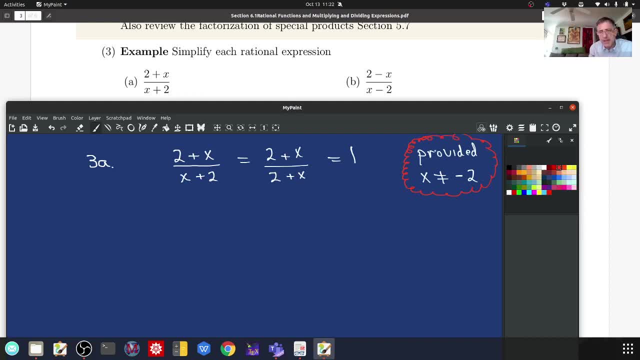 question mark. I don't think my math lab requires that you add this information. that's a criticism of my math lab on this point. you should add this information, but I don't think you do, because it's equal to 1 if, and only if, X is not equal to minus. 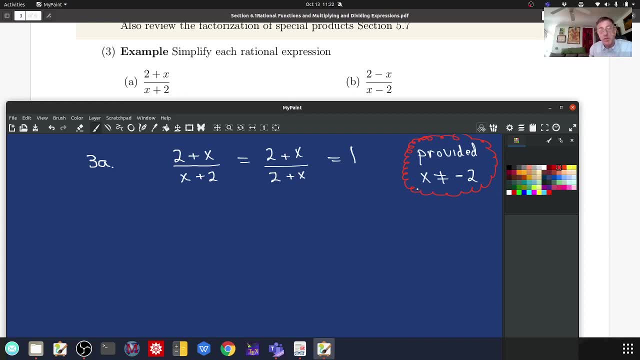 2, because if X is equal to minus 2, the whole expression is undefined. so now let's do 3b, so 2 minus X over X minus 2. now notice this is subtraction, so we don't have a commutative property of subtraction. it's not true in general. 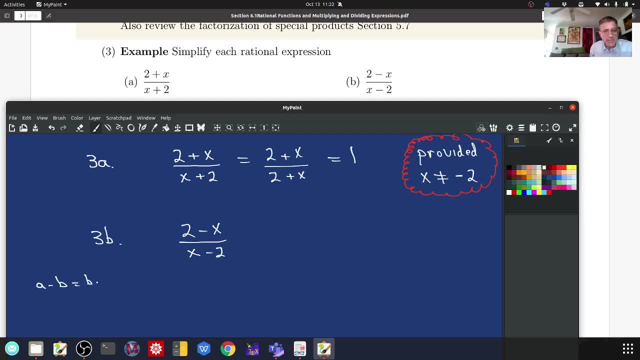 that a minus B is the same as B minus a. you want to check me on that? is 5 minus 3 the same as 3 minus 1, 5? they're not, but they are related. 5 minus 3 is equal to 2 and 3 minus 5 is. 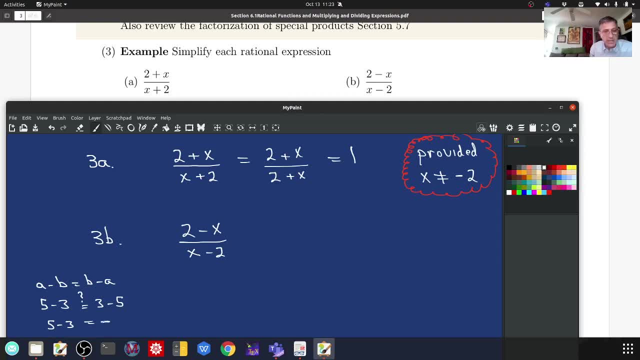 equal to minus 2. so 5 minus 3 is equal to minus 3 minus 5, and we're actually going to use that right now. 2 minus X, that's fine. X minus 2 is equal to minus 2 minus X. so just multiply that: n minus 1 times 2 is minus 2 minus times minus X. 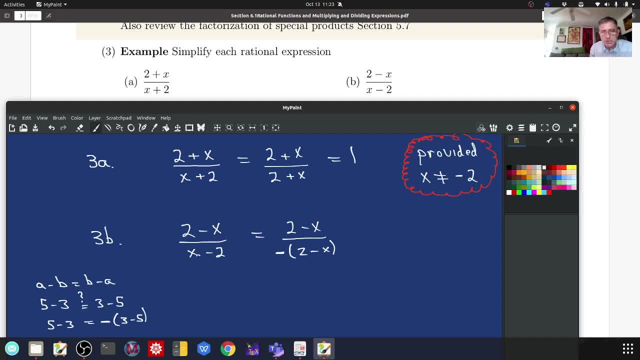 is X. so if you need to, what cancels out here? I'm going to put what cancels out here. I'm going to put put what cancels out here. I'm going to put put this here in its full glory. I'm going to fill in all of the details. 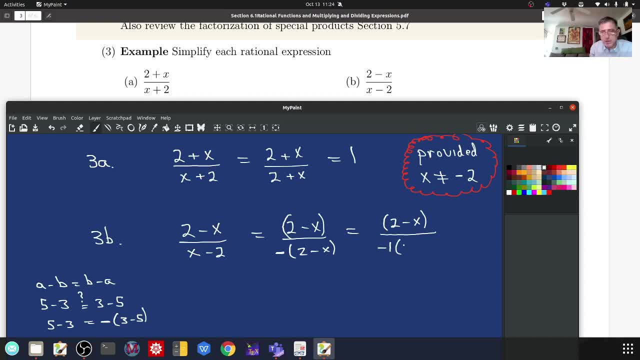 That's times minus 1, and that's a 2. there It kind of looks like a z. I'll make it look more like a 2 there. So what factors cancel out The 2 minus x factor And they become 1's. 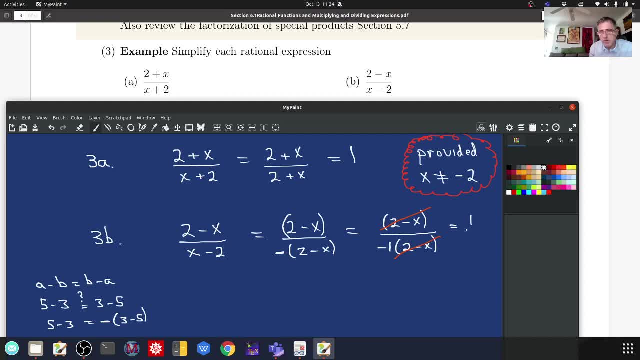 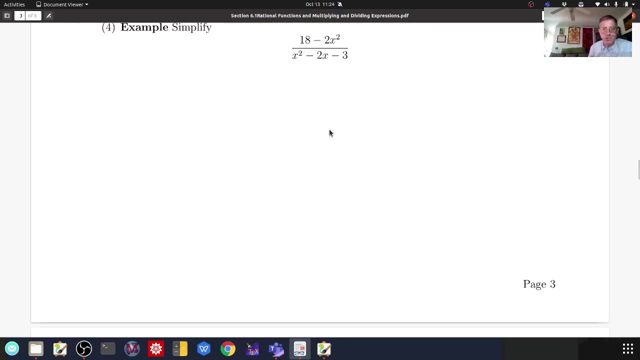 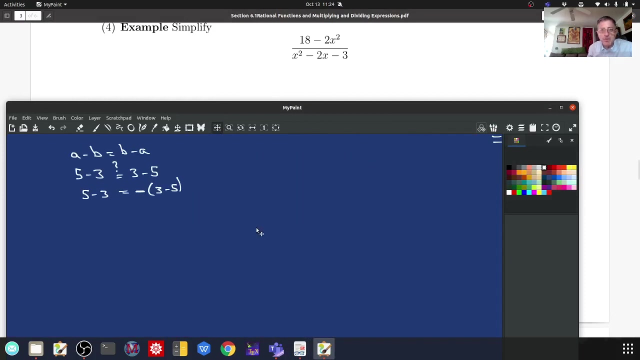 So this is equal to 1 divided by minus 1.. But that's just equal to minus 1.. So be careful there. And here's another one. I have a feeling it's going to be the same. I'm going to have to use those factorizations at some point. 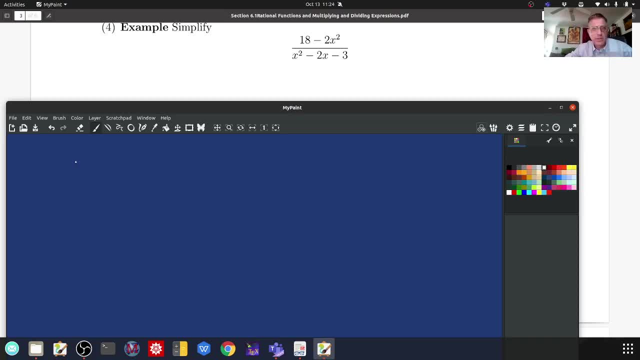 What is this one? This is just example 4.. So, Just example 4.. There is no a or b, So I'm going to challenge you to pause the video And work this one out on your own. So I'm going to help you out. 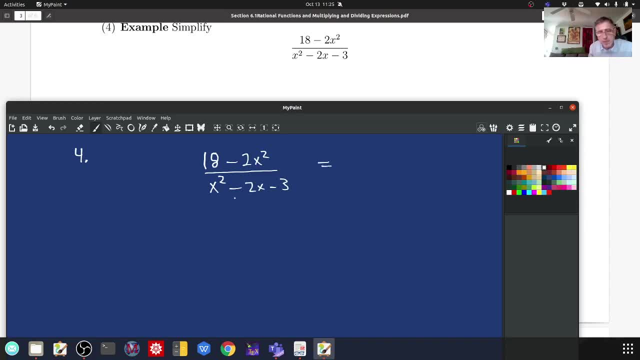 The numerator: we can factor out a, 2.. And the denominator: we're going to have to factor it. It's just a degree 2. 2 polynomial that we want to factor. So go ahead and try to do this one on your own. 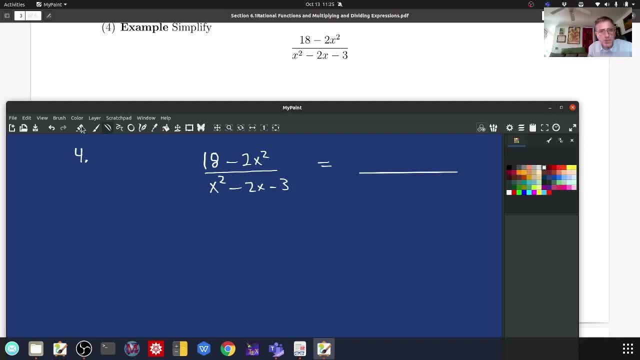 So hopefully you paused it And now you're unpausing it. So we're going to factor out a 2 from the numerator. So 18 divided by 2 is 9. Minus 2.. X squared divided by 2 is minus x squared. 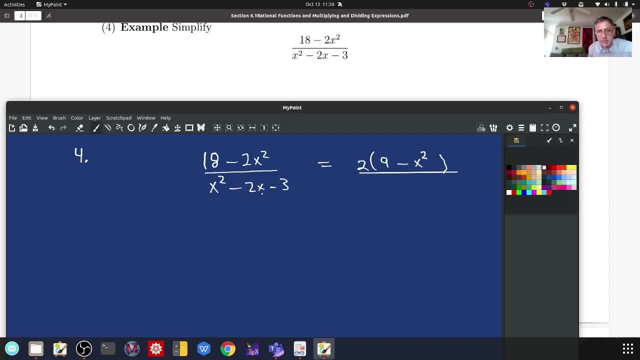 And it turns out that the factorization of x squared minus 2x minus 3, that's something you should be able to do- is x plus 1 times x minus 3.. You're going? whoa, I can't factor that. 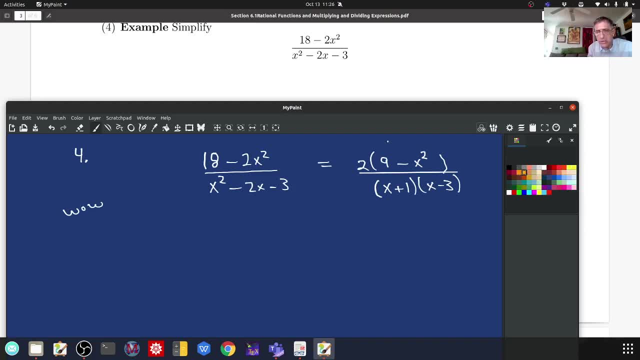 But let's take a Closer look at this factor right here. So 9 minus x squared is the same thing as 3 squared minus x squared. Oh, that's the difference of square factorization. So that's 3 minus x times 3 plus x. 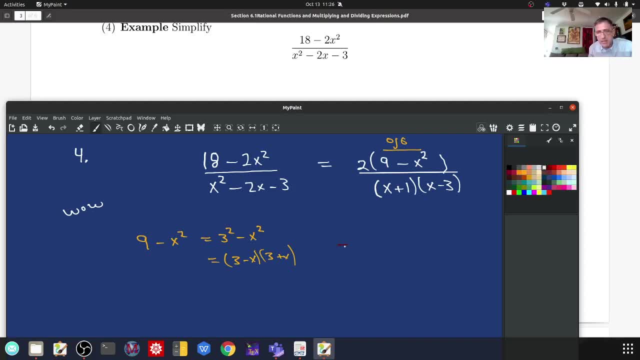 So let's go ahead and add that into my formula, Into what I've written down. So that's 2.. And 9 minus x squared is 3 minus x times 3 plus x, And it's all over x plus 1 times x minus 3.. 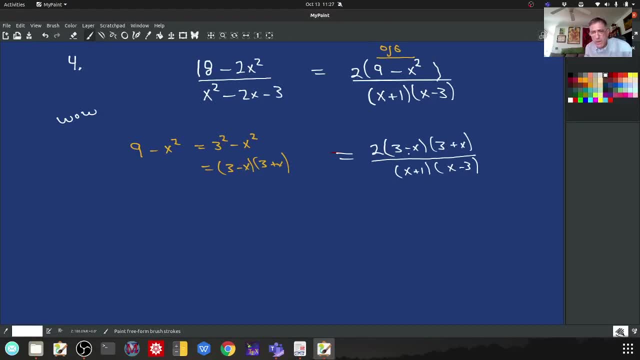 Well, it's still something's still wrong, Because if I'm looking at something, if I'm looking at a, let's say a square, Let's say a square, Let's say a square. So notice my list. first thing, let's notice. 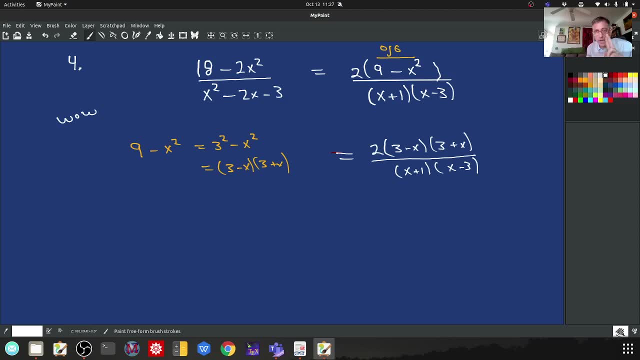 My numerator is 3 factors 2 times 3x, 3 minus x times 3 plus x. That's one thing times another thing times another thing. That's what I mean by 3, the product of 3 factors. 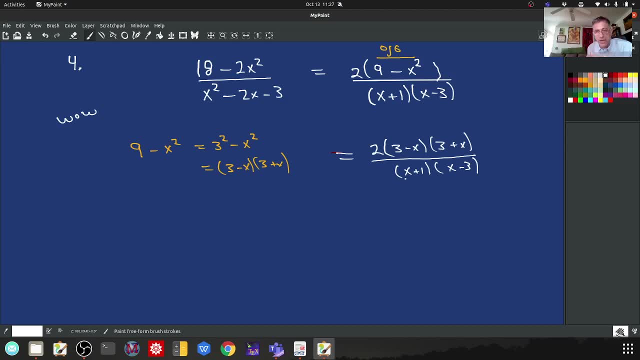 My denominator is the product of 2 factors. One factor is x plus 1, and the next factor is x minus 3.. The only candidate And the only candidate for similar factors is 3 minus x and x minus 3.. So if I negate x minus 3.. 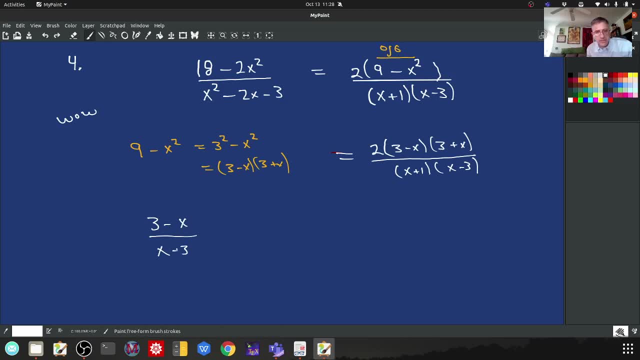 If I want to write this, what I notice is x minus 3, is equal this, But my moderator is x minus 3.. I've written down my numerator. I then take x minus 3 and lessen the denominator Okay sign. here I'm going to factor out a minus 1 from the X minus 3 term, so let 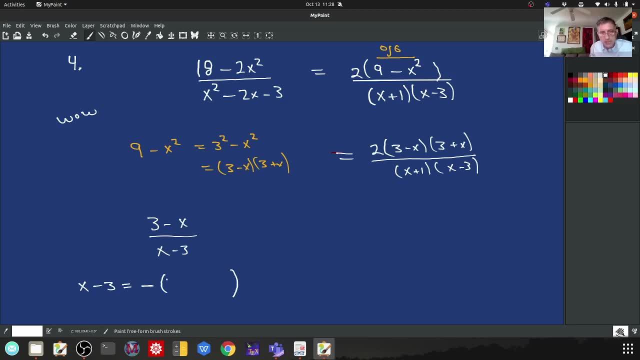 me show you this explicitly. so I write two parentheses, write a minus 1 in front of it, then I change the X to a minus X and minus 3 to a plus 3. that still doesn't look like what anything. I have but notice, if I rearrange, this is plus. 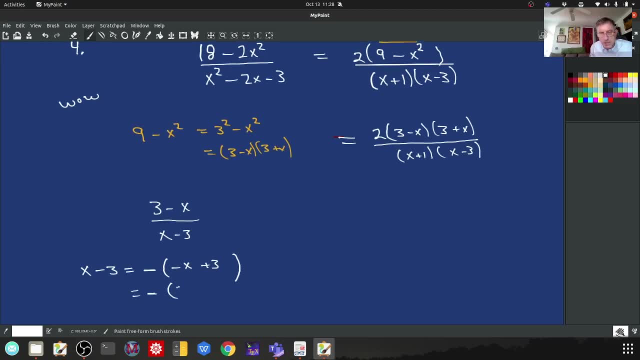 here. so minus X plus 3 is the same as 3 minus X. Wow, so this is the same thing, is two times three minus X times. three plus X times is over, sorry, divided by times. so there's three minus X and the 2 is here: 2 minus X. all right. 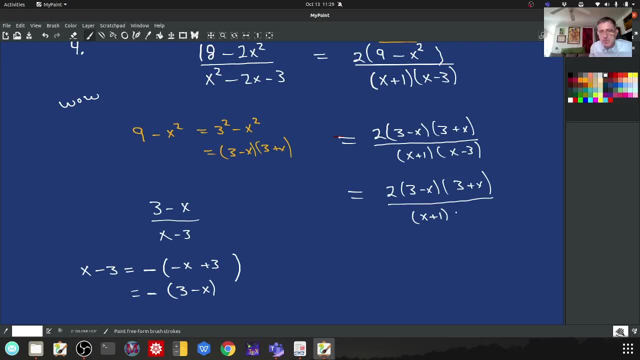 and there is plus 1 and divided by Rubik, so we get 4 times 3 plus 3, so this is by X plus 1 times minus 1. here's my minus right here. so since minus 1, since this is all multiplication, I'm going to put the minus out here in the front 3. 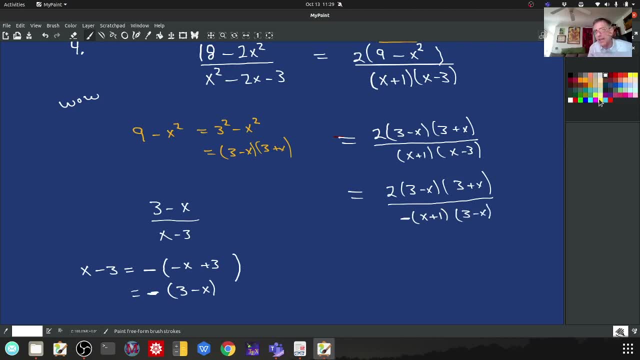 minus X. now I can actually cancel some factors- just 2- and the only thing that gets cancelled is the 3 minus X and the 3 minus X. so the customary way to write that is only have one negative and that's in the denominator. so I'm going. 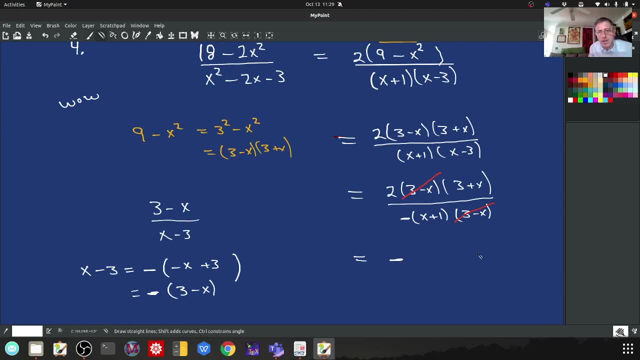 to put it right out here: even with the division line, if you've got good mathematical typography typesetting- rather it will look like that way- then I'm going to write what does not get cancelled in the numerator and the denominator and the minus. remember I've already put up here on the front, more or less in: 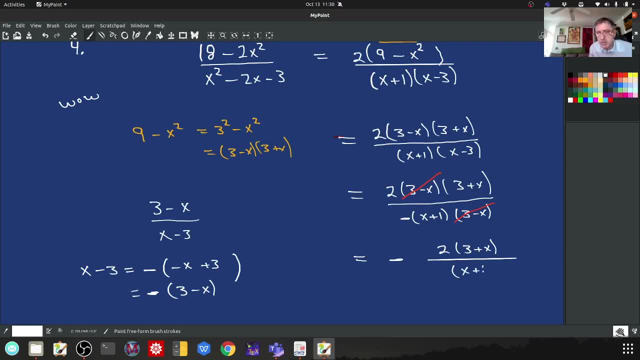 line with the division sign X plus 1. now, the X plus 1, since it's its only factor. I don't necessarily have to put those parentheses there, but you can, and that's just totally a matter of your own preferences, and sometimes I think it's better to remove the parentheses, but in this case I 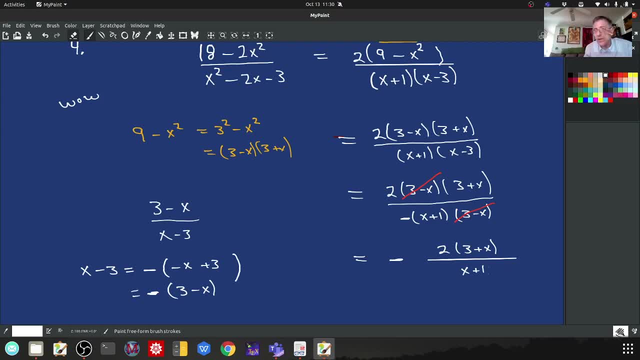 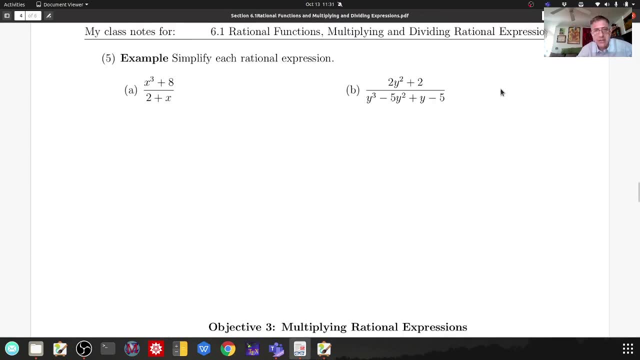 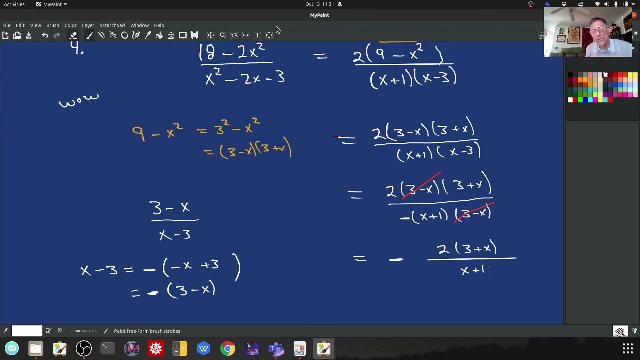 kind of like them to be there. I don't know they're. they're mathematically equivalent, so it doesn't matter. so here we're going to simplify each rational expression. so I'm going to do you the first one. for you it's important, i'm. 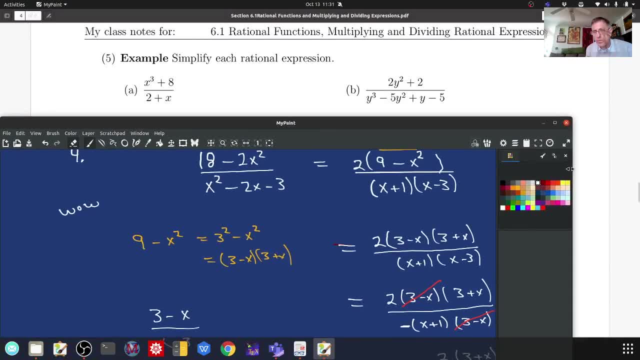 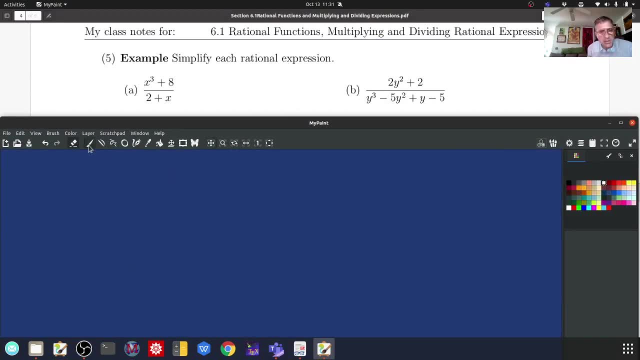 not going to test you on this one, although it's an important thing that you're aware of its factorization. so the first one, this is five a is X. notice this is a q plus eight over 2 plus x. So this has to deal with our factorization of a cubic And what I'm going. 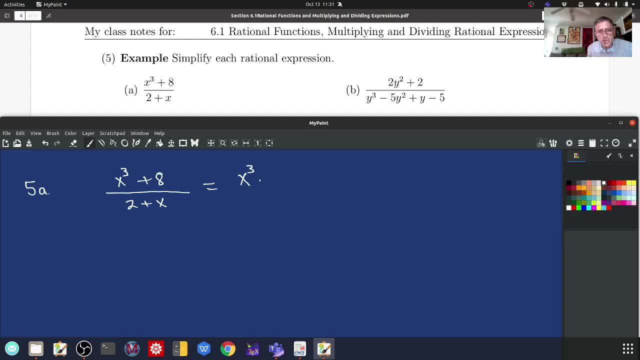 to do, to remind you, is x cubed is to recall that 8 is the same as 2 cubed. So we have to go back and look at our notes and see the factorization of the sum of cubes. So it's x plus 2 times x. 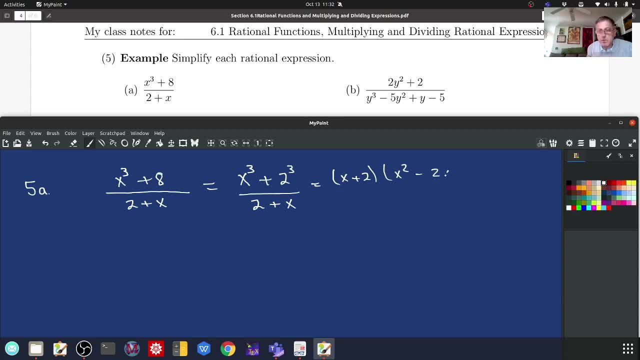 squared minus 2x plus 2. squared all over 2 plus x. Now I'm going to be lazy here. I think you've reached a step. I'm going to be lazy here. I'm going to be lazy here. I'm going to be lazy here. 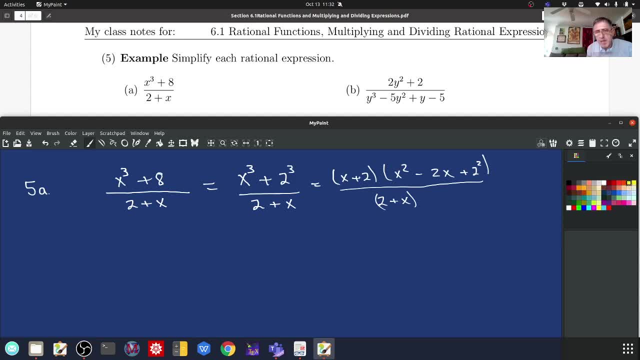 You should be okay with this. x plus 2 is the same as 2 plus x, So I'm cancelling them. That leaves the denominator equal to 1.. So my final result is: I'm just going to simplify x squared minus 2x plus 2 squared to obtain x squared minus 2x plus 4.. The only simplification. 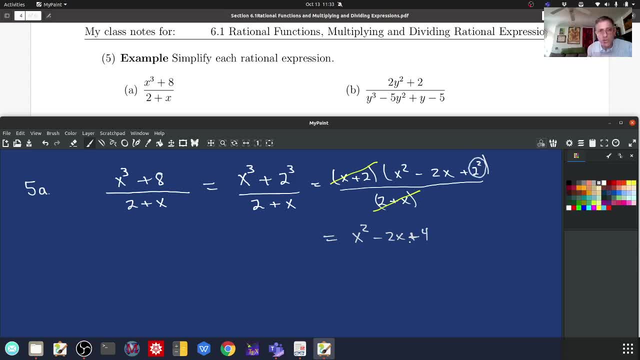 was writing: 2 squared is 4.. So this is required factorization formula. I don't recall which section it was in. I think it was in chapter 5.. What section? Maybe 5.5.. The factorization formula for sum of. 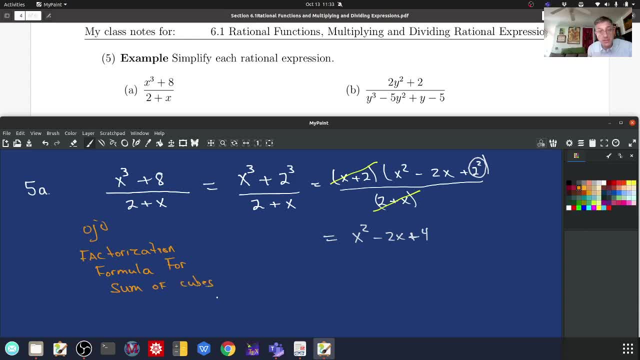 cubes. There's also a difference of cubes, but this is a sum of cubes And 5b. Now this is an interesting one too. So I have 2y squared plus 2.. So I hope you're immediately saying I can factor out a 2 from there. 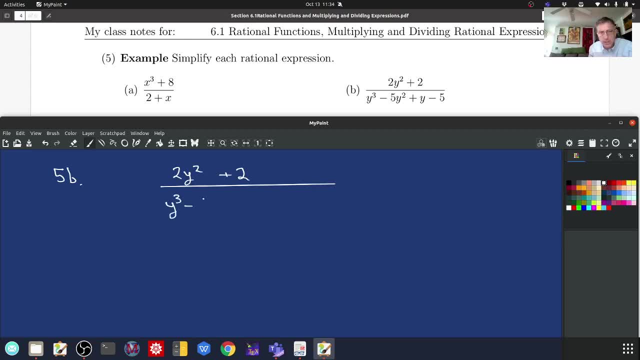 But this bottom one is a cubic polynomial. in the variable y It's not the sum of 2 cubes, because y is the sum of 2 cubes. So I have 2y squared. There's just a sum of more than 2 things. 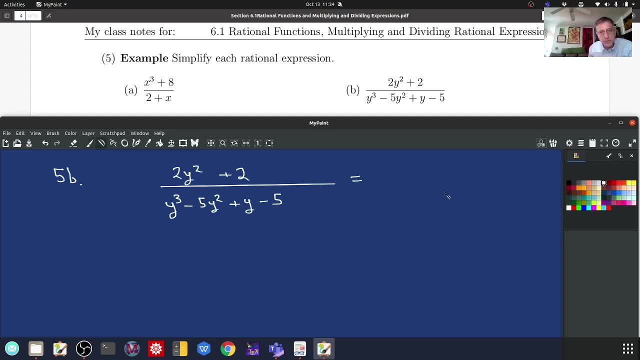 So we're going to have to use some tricks here. Let's just do the most obvious. Let's factor out a 2 from the numerator. So 2y squared divided by 2 is y squared, And 2 divided by 2 is 1.. 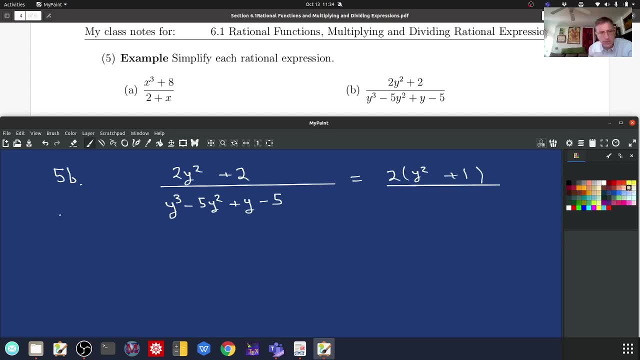 Here, the only thing I can invite you to do is to write the sum of 2.. What I'll write you to note is there are 4 terms, So we have had instances in the past where we can factor 4 terms like this by grouping: 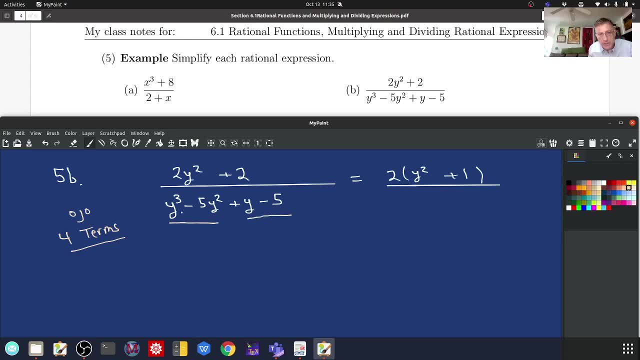 So what I'm going to do is I'm going to factor out the greatest common factor of this 1st group. So the greatest common factor of y is 1.. greatest common factor of y cubed and 5y squared is y squared. 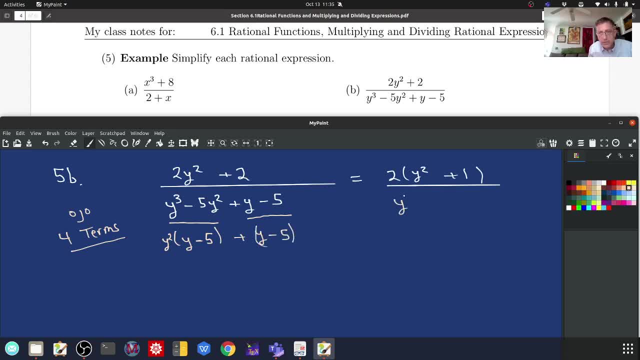 Okay, so I'm going to write it that way: Y squared times, y minus 5.. A similar question was on the exam or a factorization of this form, and I'm going to continue on Now. some of you are already smart enough to realize that the 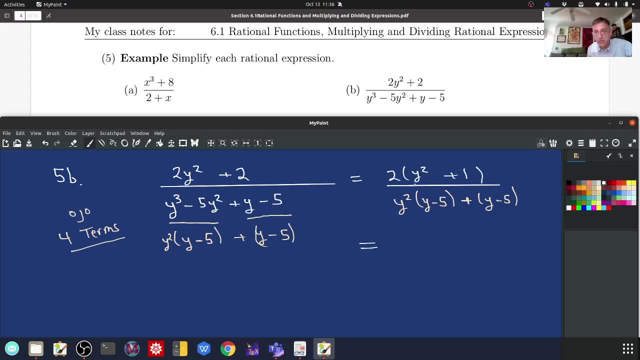 end result is probably going to have y squared plus 1 as a factor somewhere. So we don't have it anywhere right now, but notice that this is plus 1 times y, squared y minus 5.. So if I look at these two terms, this is one term and this is. 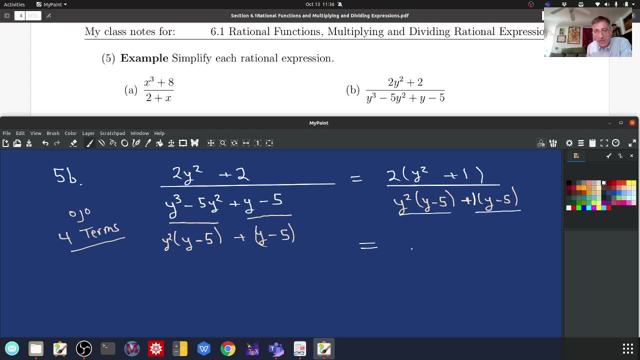 another term. they have a common factor, and that common factor is y minus 5.. So I'm going to factor out y minus 5.. So y squared times: y minus 5, divided by y minus 5 leaves me a y squared. 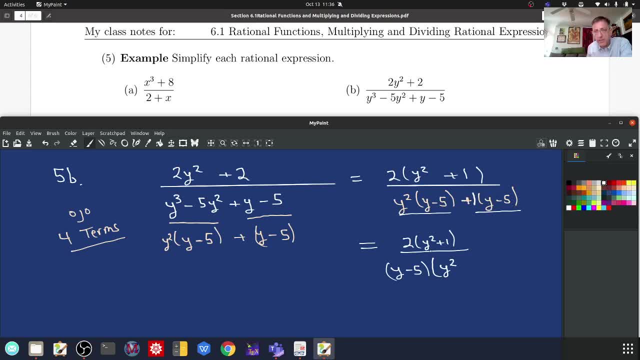 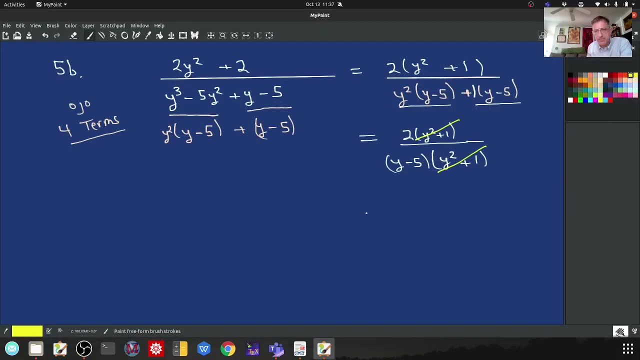 Plus 1 times y minus 5. divided by y minus 5 gives me a 1.. And finally we reach a point where we have a factor in the numerator and a factor in the denominator that are the same. So I write what I have left over. I have left over a factor of 2. 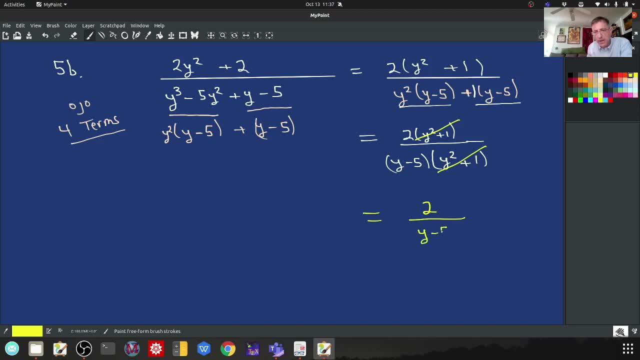 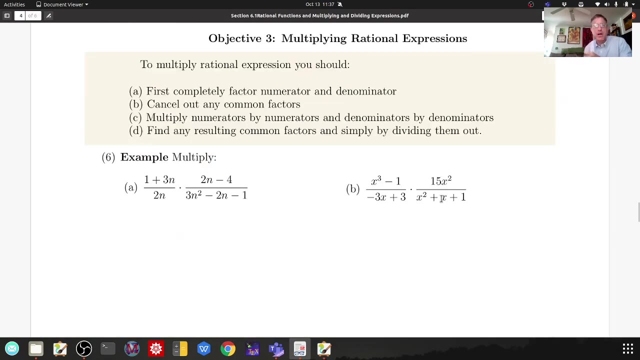 in the numerator and a y minus 5 term in the denominator. It makes no difference whether you leave it in parentheses or not. So now we're going to multiply rational expressions and then we're going to divide them. Sorry people. So for this particular part I'm going to just write: 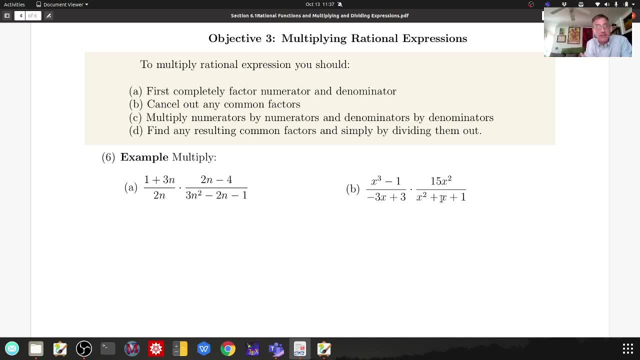 the factored form. So I'm going to write the factored form and then I'm going to write the factored form, But the factored form is better than the factored form. I'm no longer going to factor anything. I will tell you what you should do to factor. 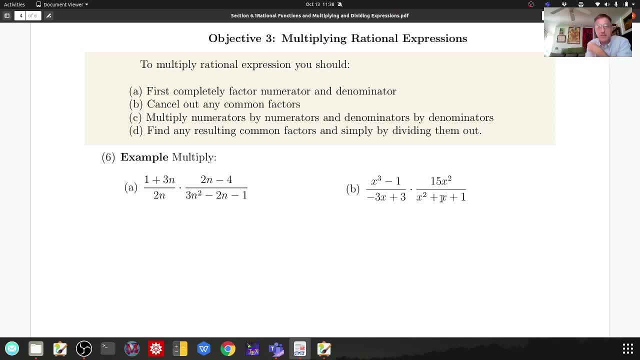 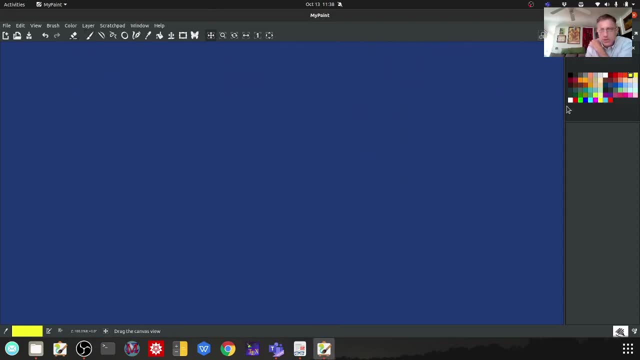 them. and that's it, Because what we're going to focus on on this part is canceling factors. So here's a skill that you should've mastered. Suppose I have x to the fifth times y to the eighth, over 2.3.. 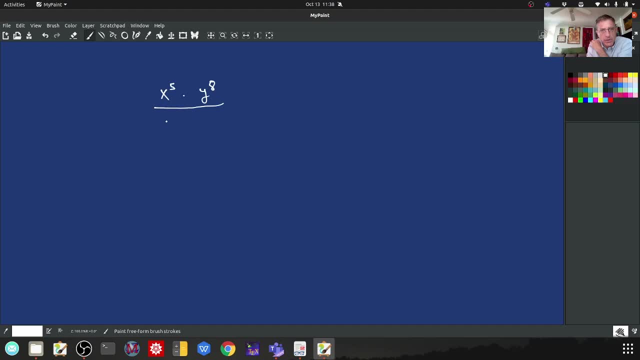 Here's the thing. I just want to write down what I've done: Z to the fourth times X. I'm hoping you're good enough now to say: well, look, here's an X to the fifth. here's five X's multiplied together in the numerator and one X multiplied. 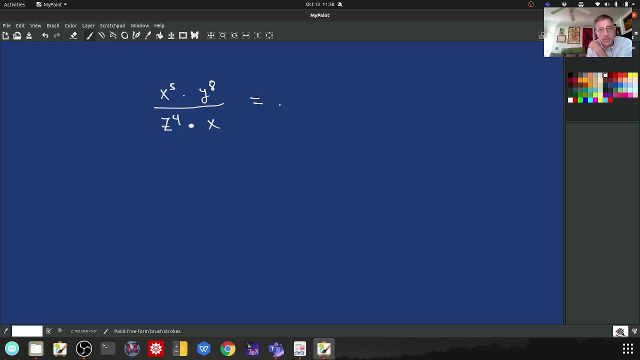 together in the denominator. So one of those X's will cancel out, leaving me X to the fourth, Y to the eighth, Z to the fourth. So in other words, you just cancel out one factor that's supposed to and X-ing out an X, it still becomes an X, So that cancels. 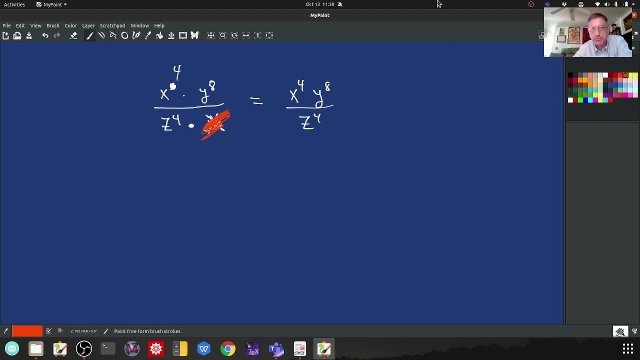 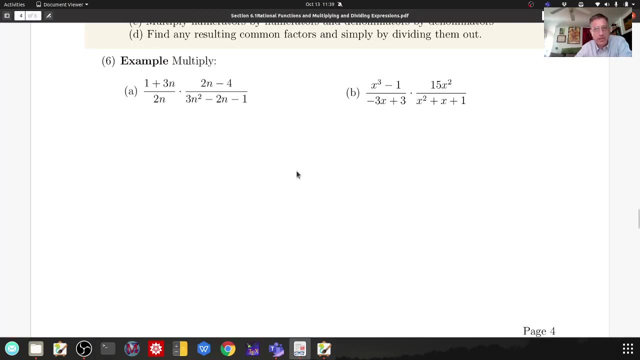 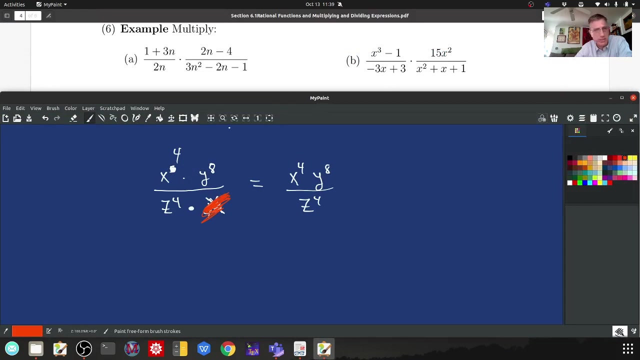 out. So we're going to be doing something similar. We're going to be multiplying and then simplifying. So right now, here is the big no-no: When you go to multiply these out, you do not use distribution. If you use distribution, you've ruined everything. So the first thing I want 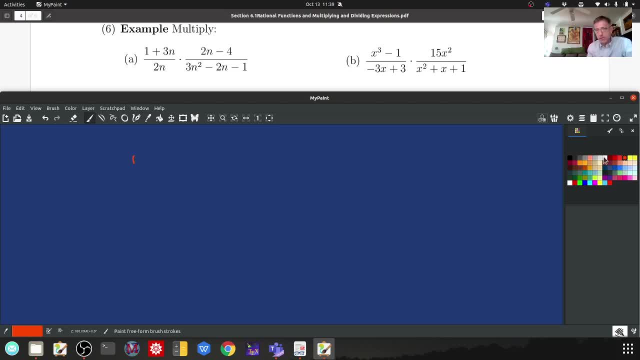 to do is change my color. This is 6A. I want to completely factor every term. 1 plus 3N is a prime linear factor and 2N is just a product. There's nothing that can be done And I'm using the dot for multiplication. 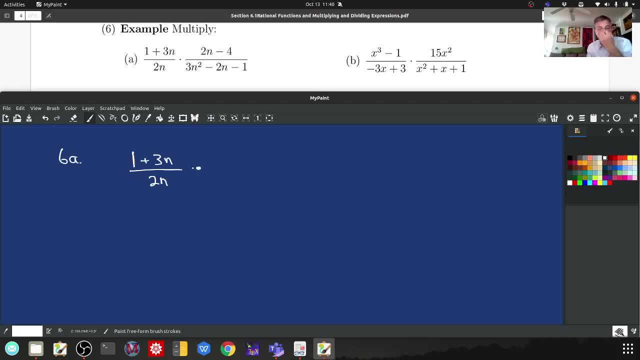 here You can also use big parentheses. So up here, 2N minus 4, I'm going to factor out a 2. That's going to leave me N minus 2.. Now on the bottom, this polynomial: when I factor it, I'm going to get N minus 1 times. 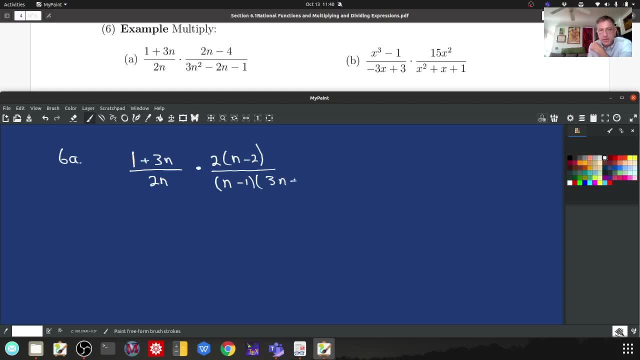 3N plus 1.. So now becomes the search for common factors. Here is a 2, and here is a 2. I can only cancel the 2., Not the N, just the 2. N minus 2, there is no N minus 2 up here. 1 plus 3N. There's not a 1 plus 3N, but there's. 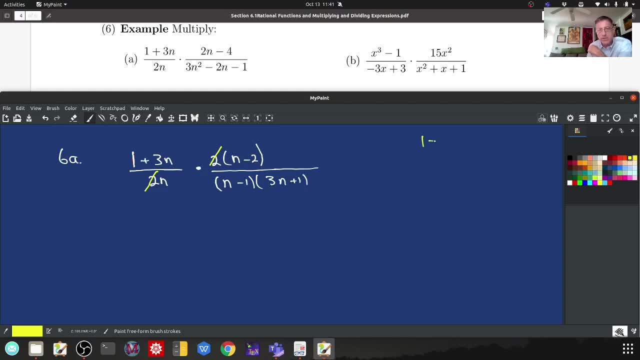 an equivalent to it: 3N plus 1.. Just remember, 1 plus 3N is the same as 3N plus 1.. Why? That's just the commutativity of addition. So these, this entire factor here, if you want to put it in parentheses- cancel And. 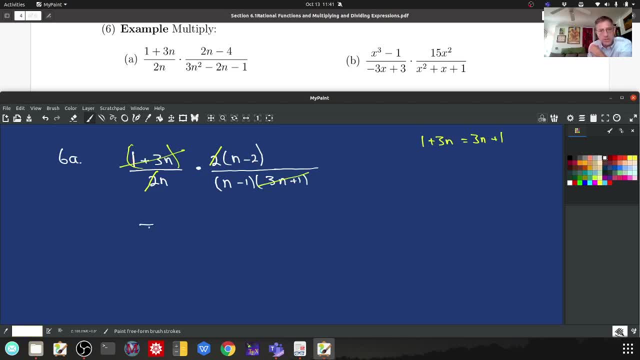 you get that one. So what do you do next? You simply write as a fraction every factor that remains. What remains in the top is an N minus 2.. And on the bottom we have an N And notice this is multiplication. So it's N times N minus 1.. And that's its simplification. 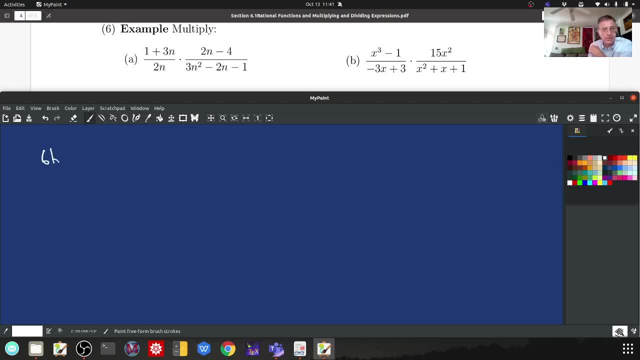 So on the bottom we have an N minus 1.. And we just cut the N and make H the same number as X cubed minus 1.. So X cubed minus 1. And that's the same as X cubed minus 1 cubed. So that means we're. 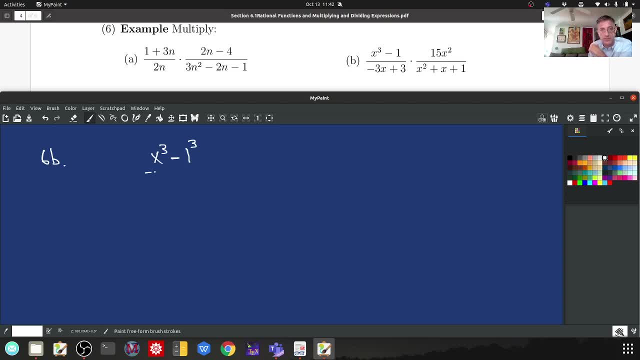 going to use the difference of cubes for that: factorization Minus 3X plus 3. And we're multiplying that by 15.. Marianne, do you want to do another one? Oh, I'm sorry. No, Come on. 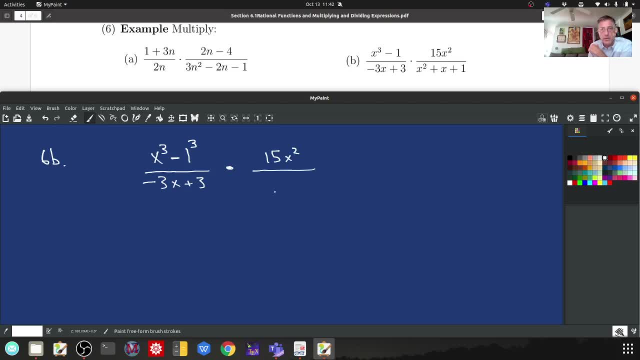 Come on: x squared over x squared plus x plus 1.. So let's start simplifying. The only thing I would think that you would need help with is this is the difference of cubes. So x cubed minus 1 is x minus 1 times x squared plus x plus 1.. 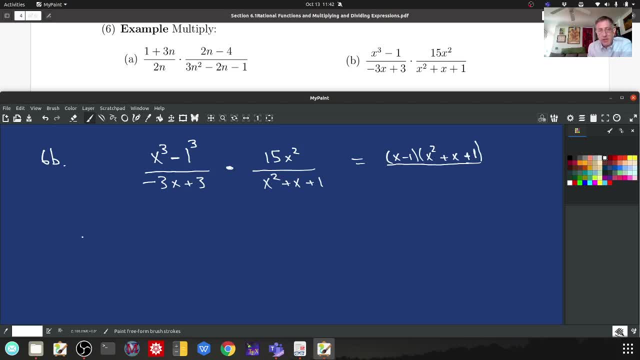 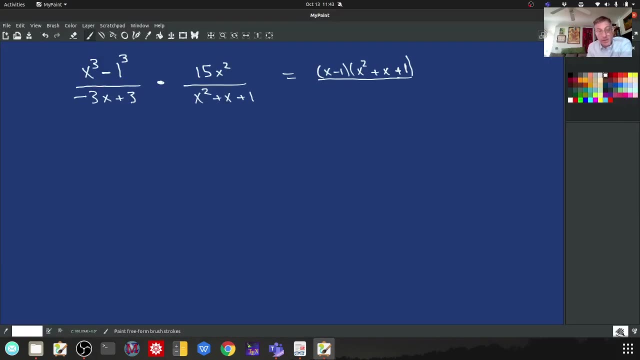 That is its factorization. If you write it as x squared minus 1 cubed, you can look at the formula. Now, let's scoot this over and give me some more room. Let me full screen here Now. here I can clearly factor out a 3.. 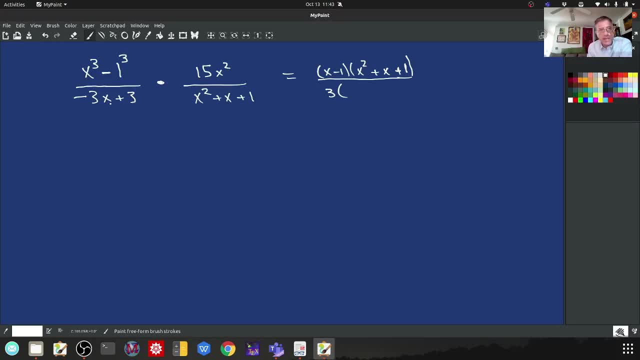 So this is going to be 3 minus 3x divided by 3 is minus x plus 1.. Now, minus x plus 1 is the same as 1 minus x And the factorization of x squared plus x plus 1 it's prime. there is no factorization of this. this is worth. 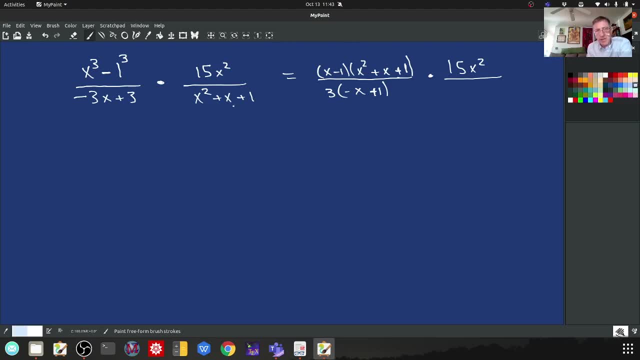 doing so, let's try to factor x squared plus x plus 1, because normally you've been dealing with polynomials that can be factored and suddenly we've encountered one that can't be factored. so let's just, let's, let's go over that. 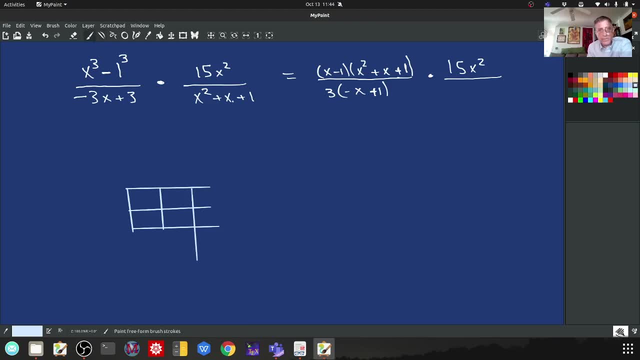 let's try to factor x squared plus x plus 1. so this is my x squared, this is my 1, this is my X. this is really easy to discover. they can't be factored, so I have to put an X here and an X here. there's no choice. so X times X is X. 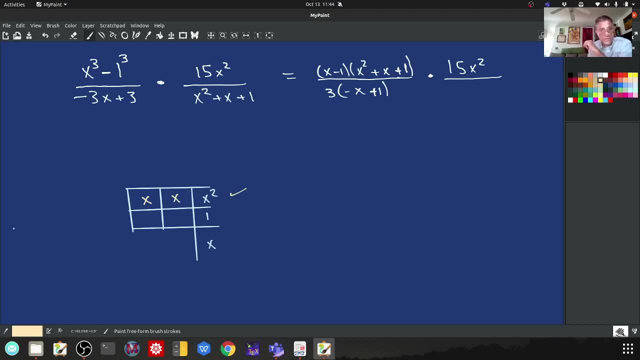 squared here. 1. I have two choices, like two choices, for 1 is 1 times 1. my other choice is minus 1 times minus 1, and we don't want to use the minus 1 times minus 1 because when you add them, 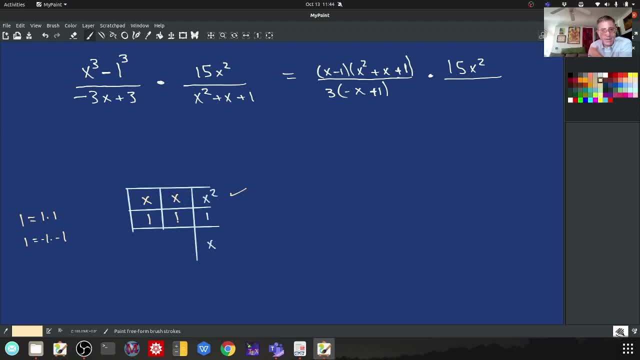 together you're going to get a negative. so I have to put a 1 there and a 1 there, so that gives me X plus X, and X plus X is equal to 2x and that's not equal to X. and if you were to do the minus 1- and you don't believe me- then I would have. 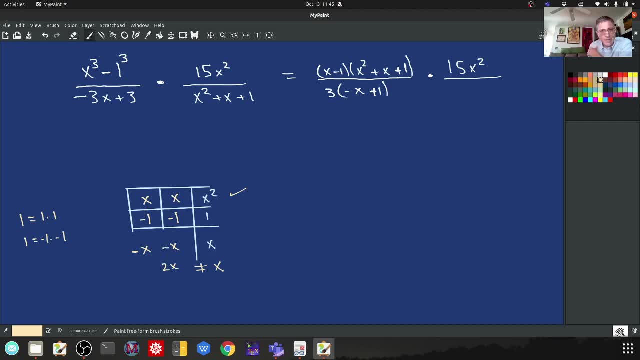 minus X, minus X, that minus 2x and that's not X. so what we conclude? we literally exhausted all of our possibilities that this polynomial is prime, so I'm going to go ahead and put it in parentheses, and the reason I'm doing that is it's. 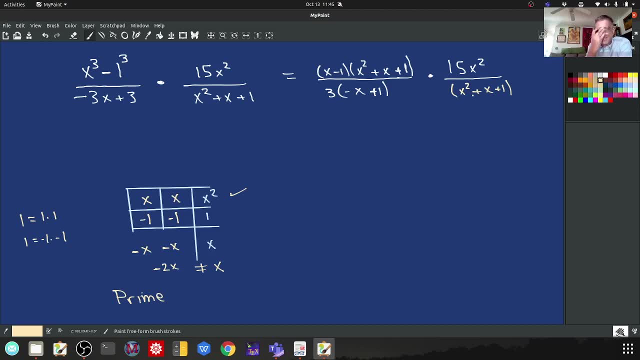 probably. if you do that, it's probably less likely that you'll make some weird mistake. so now I'm looking for like terms. well, here I have X squared plus X plus 1, so I can cancel that. 15 divided by 3 is 5, so I'm going to replace that with 5 x minus 1 and minus X plus 1, minus X plus 1 and. 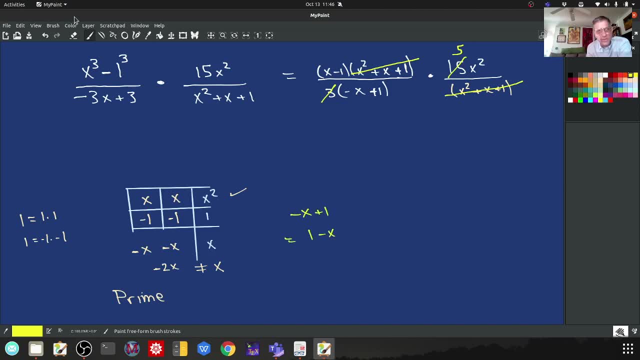 is the same as 1 minus x. So let's just write it as 1 minus x, But we still don't have x minus 1, but 1 minus x. if I pull out a negative is minus 1 plus x. 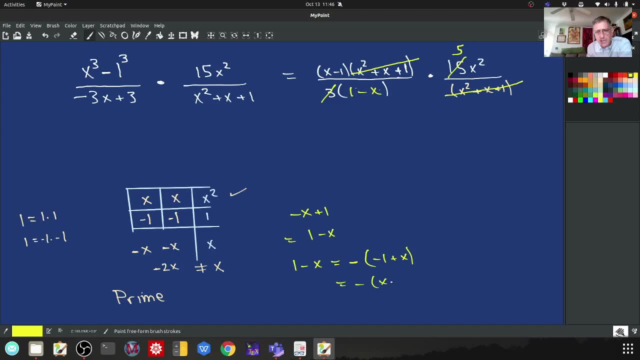 which is equal to minus x minus 1.. So let's go ahead and write that down. I probably did an extra Whoops, I didn't want to do that. This is minus sorry. I hit the control Z and erased some stuff that I'd previously written. 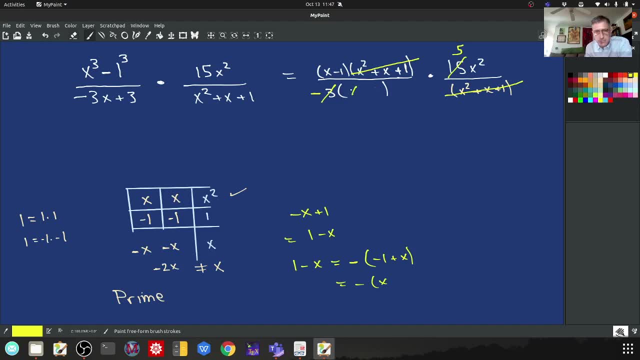 and I'm being lazy. I didn't want to do that today. Now, remember, the minus 3 has been cancelled, So now maybe I should use red to cancel things out. The minus 3 has been cancelled and the 15 has been changed to 5,. 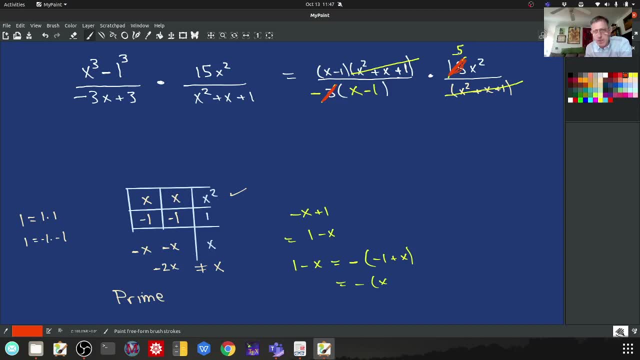 because 15 divided by minus 3 is minus 5.. I'm leaving the minus right here for right now. Then I can cancel out my x minus 1 term. Now, let's change all of this. Let's change all of this. 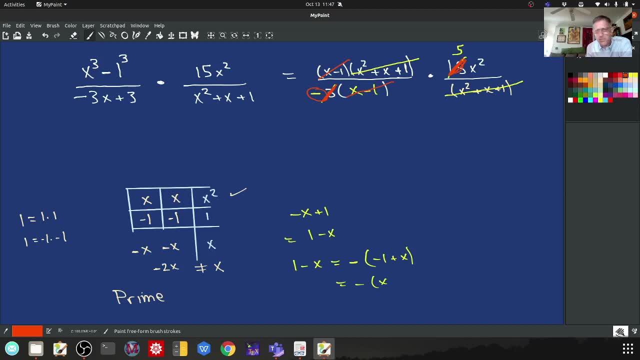 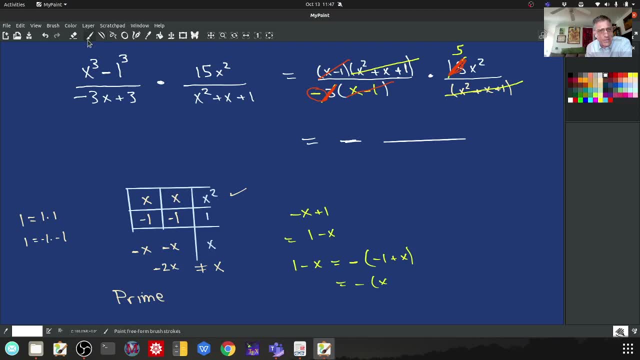 And the only thing remaining in that slaughterhouse of cancellations is a 5x squared in the numerator and nothing. Everything was gone in the bottom. So you can put a 1 here- and that's just going to simplify- to minus 5x squared. 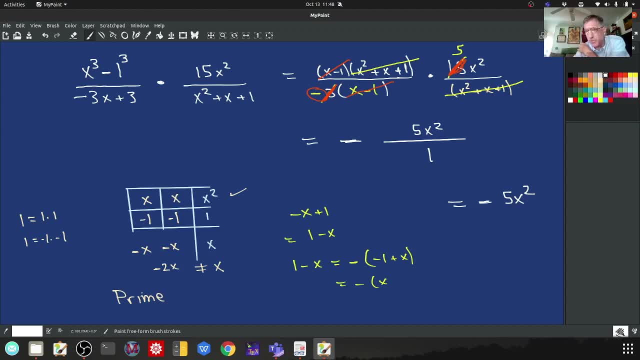 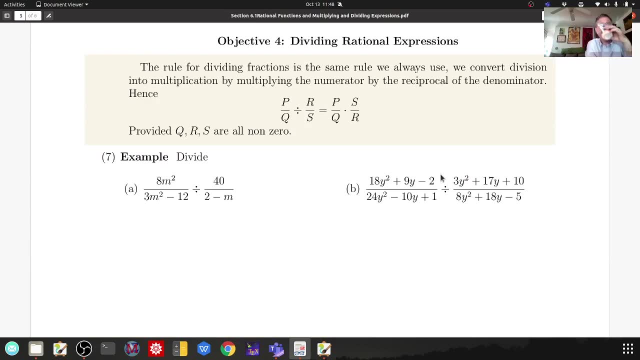 So these are some really good examples. Now here's the thing about dividing. So the rule for dividing tractions is is the same rule we always use. We can divide two fractions by converting the division sign right there into a multiplication sign. 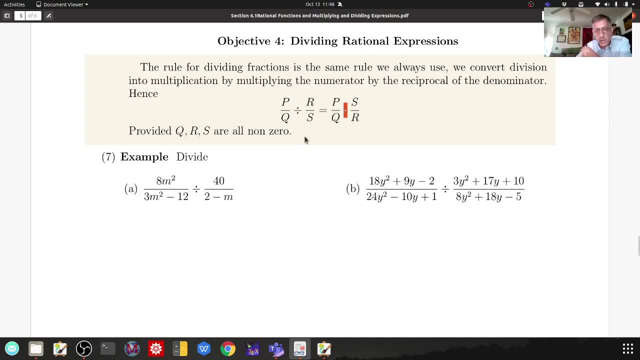 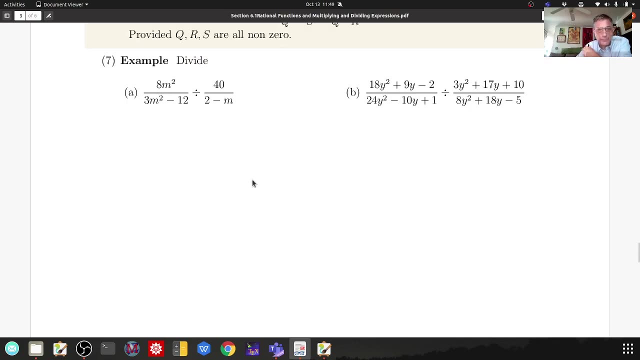 Multiplication of fractions is super simple. We have to pay a price for that conversion, though, So the r divided by s turns into its reciprocal s divided by r. That's all there is to it, So let's do this. 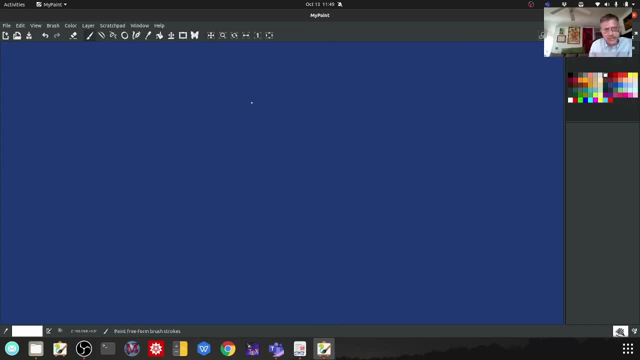 If you're ever given something like this- a divided by b over c divided by d- you can always figure out what to do. For those of you who know the invert and multiply, I'm going to give it to you right now. So there's two ways to do this. 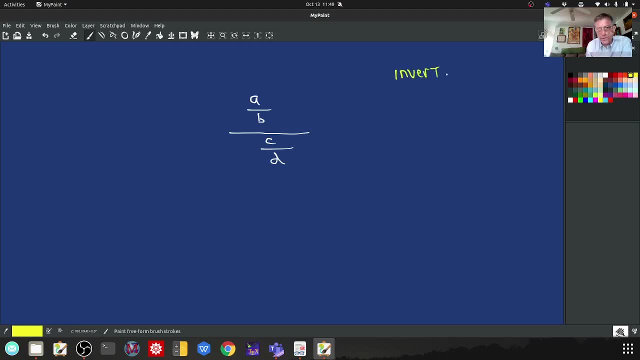 One is called invert and multiply. This should be a review. Well, what gets inverted? Remember, this is my denominator, right here, My denominator is a fraction. So I take my numerator, which is a divided by b, invert and multiply. 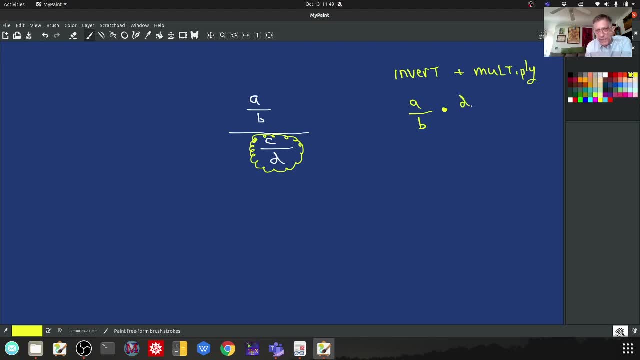 What gets inverted? The c divided by d, And it becomes d divided by c, And that's a d over b c. Another way to figure out what to do is just write what this says. This says: divide a divided by b. divide it by c divided by d. 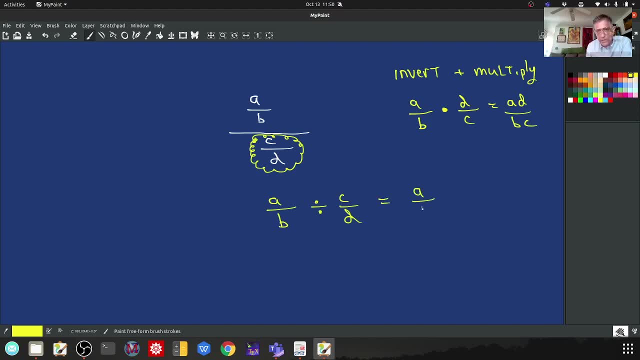 Well, I can just change the division sign into a multiplication sign, but the price I have to pay is: invert the c divided by d And lo and behold, it's exactly what I did up there And you get the exact same thing. 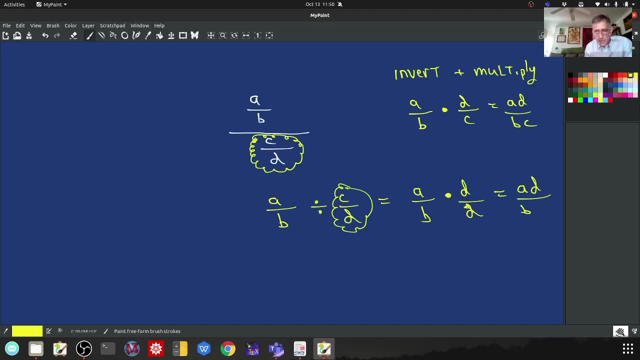 Oh well, it would help if I inverted it right: C divided by d inverted, is there we go And we got the exact same thing. So that's the technique we're going to use, And as soon as we do that, we're already back one step. 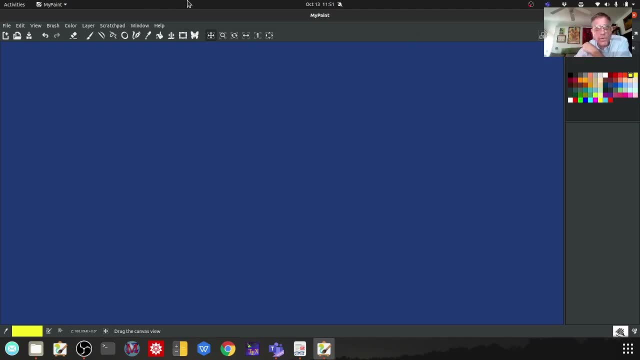 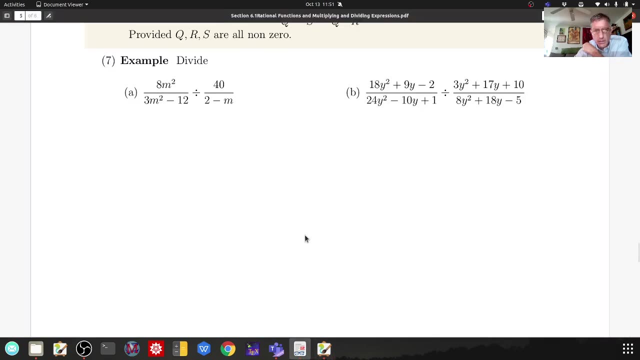 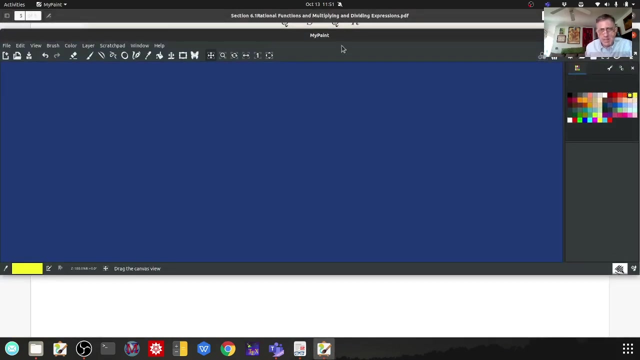 We, we, we've, we're back to what we were doing before simplifying multiplication. I don't want to show you that, So I'm going to do these again when we get to number one, Number b. I'm not going to do the. I mean just to keep this lecture at a reasonable level. 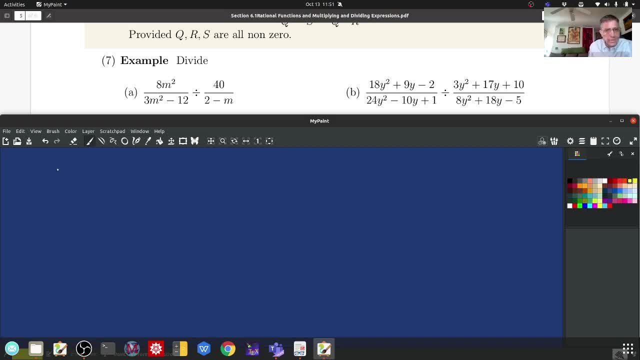 You. I know it's not true, but in the ideal world you should already know how to factor all of these trinomials, And indeed you can. So I'm going to factor them for you And when you're doing the work. 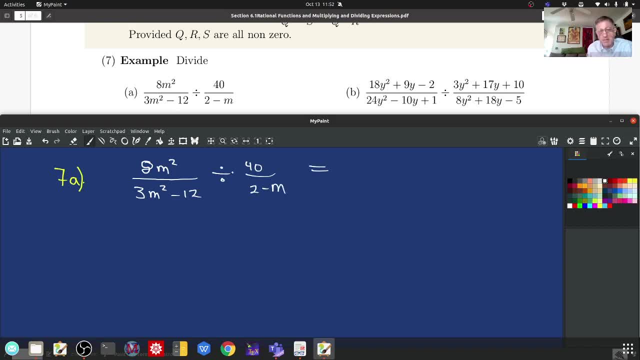 you can check it or do it on your own. So the first thing I'm going to do is I'm going to change this back to a problem of multiplication. So my numerator is the first, So I'm going to do a fraction here and this is going to be changed into multiplication. 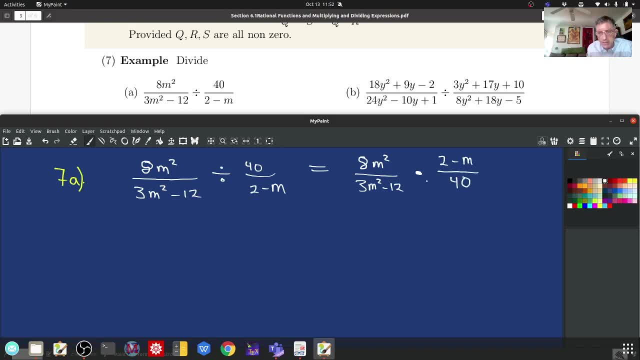 by inverting this fraction. Now, let's go ahead and work on this. We'll go ahead and put this in parentheses. I sense that might be helpful. The only thing that I can factor here is this term: 2 minus m is a prime, is a prime linear factor, because 2 and m don't share any common factor. 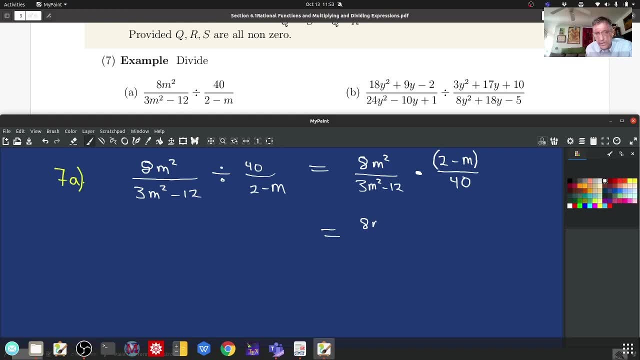 But 3m squared does share the common factor of 3.. So I'm going to factor out the 3 and get m squared minus 4.. Times 2 minus m over 40. Well, I'm expecting a little bit more about that. 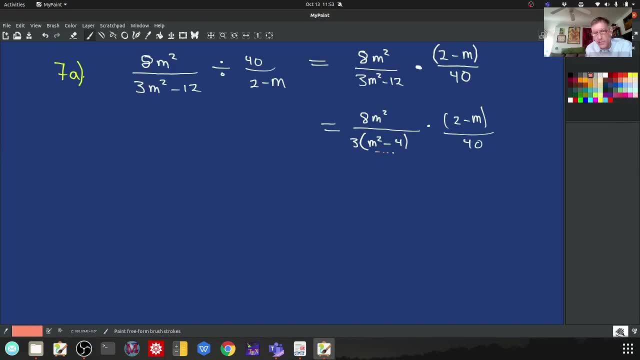 And I should be able to do more, and indeed I can. So let's go over here and look at m squared minus 4.. Well, m squared minus 4 is really m squared minus 2 squared, And that's one of those special products. you just have to know. 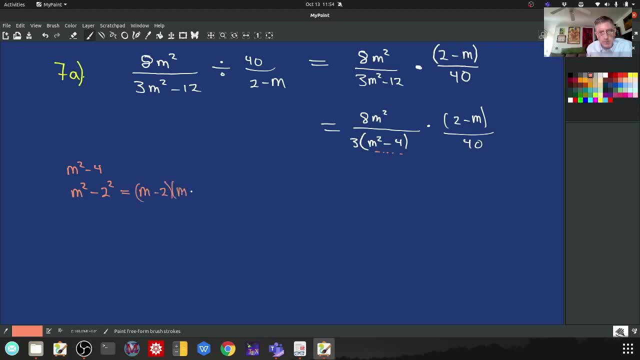 That's m minus 2.. So instead of: I'm going to be super lazy here and I'm just going to rewrite this as what it's supposed to be, That's m minus 2.. Well, I guess I'll use m minus 2.. 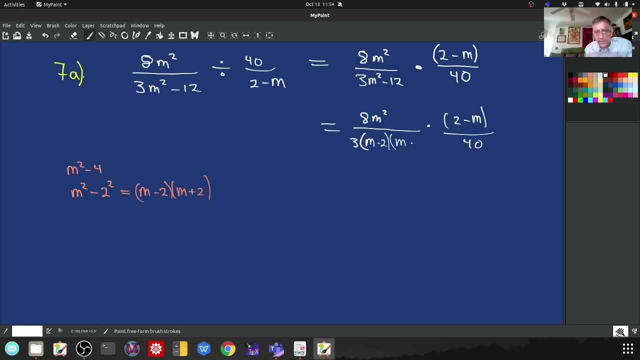 And that's m squared. So instead of- I'm going to be super lazy here- Times m plus 2.. And aren't you aggravated Because here I have a 2 minus m? But 2 minus m is equal to minus m plus sorry, m minus 2.. 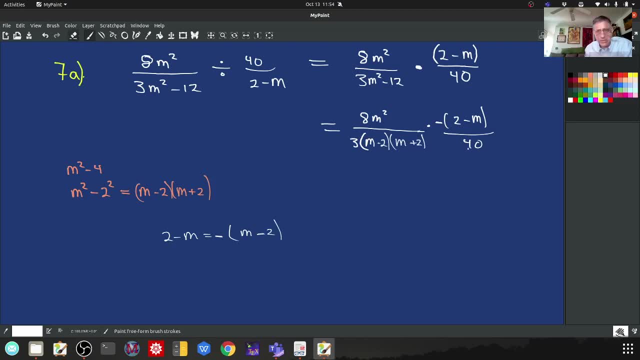 So I'm going to change this to again. just being super lazy, I just don't want to rewrite that. I'm going to rewrite this entire line. It's one of the things I do wish this program had. I wish it would allow me to cut out something and paste it someplace else. 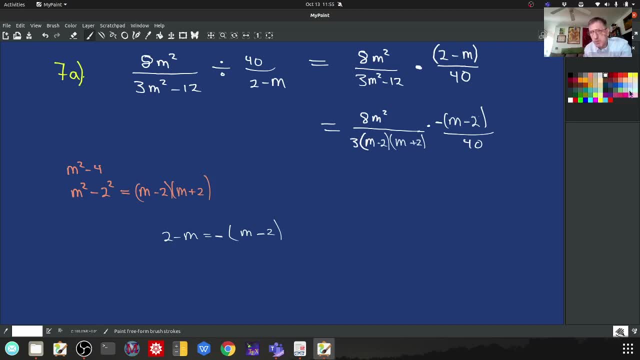 And it doesn't have that feature. But it's really simple and it seldom crashes and it uses. it loads up fast, And so here is m minus 2. So just be careful. The only thing I'm factoring Can't do that. 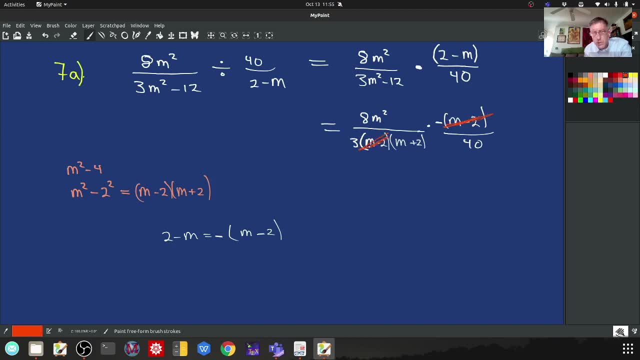 Canceling is the factor of m minus 2. The minus stays, And then the 8.. 8 divided by 40 is the same as 1 over 5. Because 40 is equal to 8 times 5.. So just to let you see this right here. seems magic, but not really. 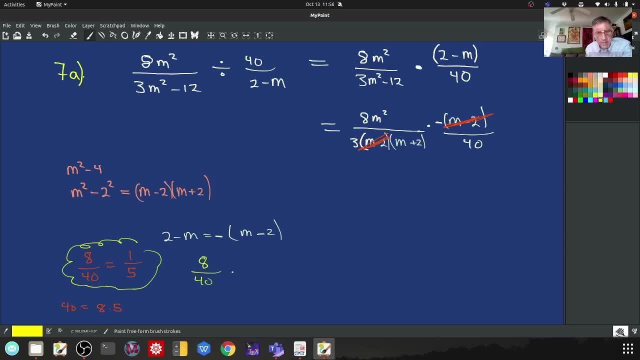 8 over 40 is equal to 8 over 8 times 5.. So I'm canceling the 8s. That gives me 1 5th. So I'm going to change that to 1 and change that to 5.. 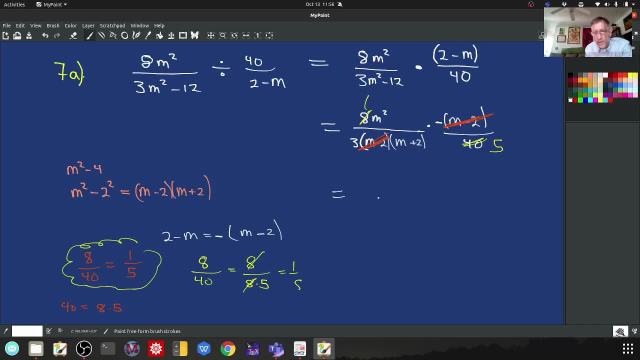 And I think that's everything that we can do. So I'm going to. I have a minus, just one minus, in there. If I had another minus, they would cancel each other out, And if I had a minus, that would cancel each other out. 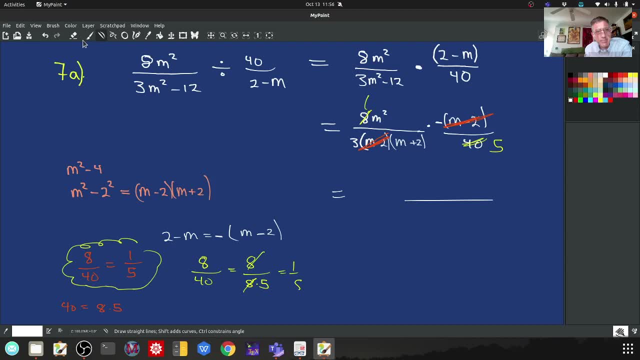 So I have an m squared in the top. I've put my minus in this out here. then I have a five in the bottom times three. so here are my constant terms: there's a five and there's a three times m plus two. 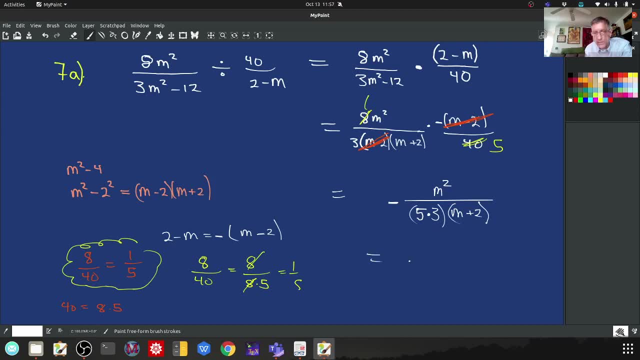 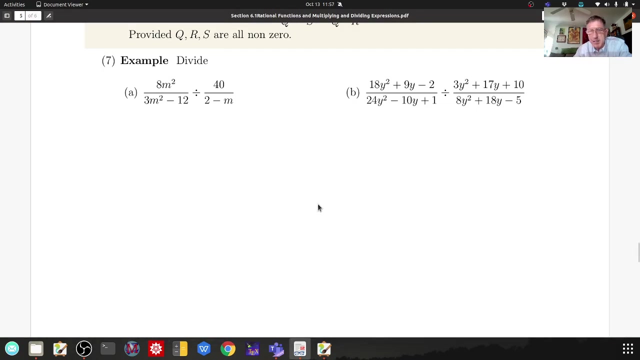 Those have to be in parentheses. so that's equal to minus m squared over 15 times m plus two. I extended the division line further than I needed, Okay, so let's do this next one. It looks really daunting, but we need to do it. 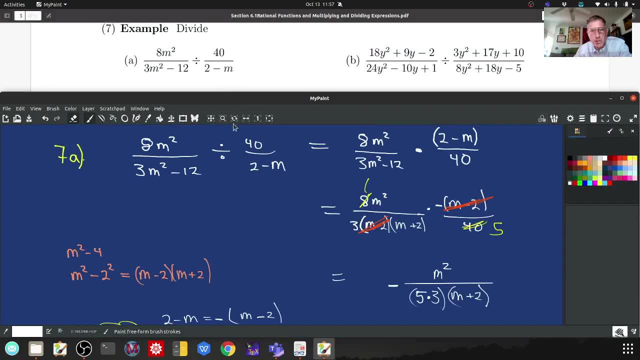 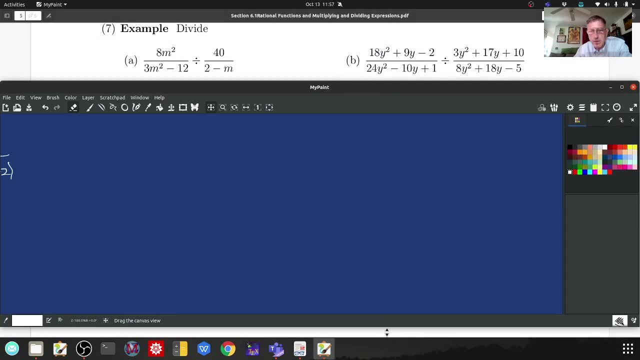 But really the only thing for this next one is the need to factor everything. There's four polynomials that you have to factor, And what I'm going to do is I'm going to do this. Okay, Okay, Okay. I'm literally just going to write down their factorizations. 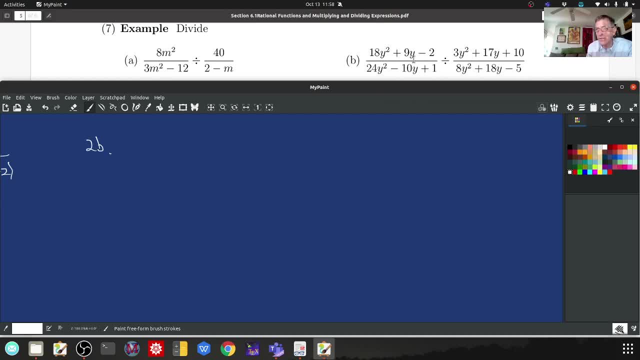 So 18y squared plus 9y minus two becomes 6y minus one. I'm not doing this in my head, I have it written out. I've done the work on all of this before. Three y plus two. So if you multiply that out, 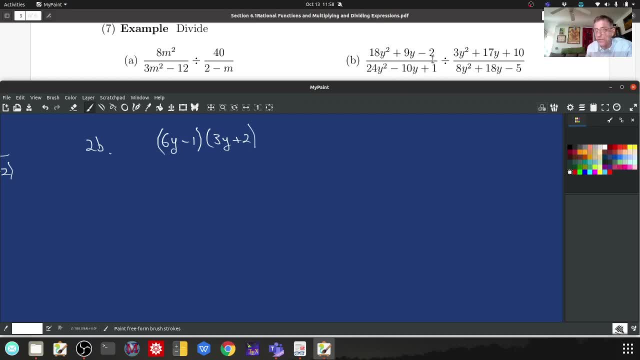 You'll get 18y squared plus 9y minus one, 24y squared plus 10y plus one. So there's, you can only factor it, I mean there's no common factor there. Then when you do it, thankfully you're going to get a 6y minus one times 4y minus one. 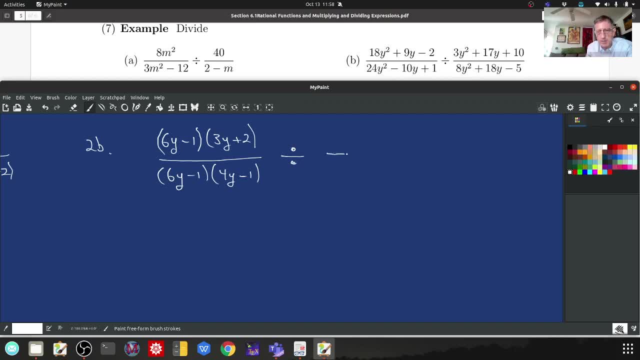 This is going to be divided by Doing the factorization first. So 3y squared plus 17y plus 10.. That's y plus five Times 3y plus two, And 8y squared plus 18y minus five. 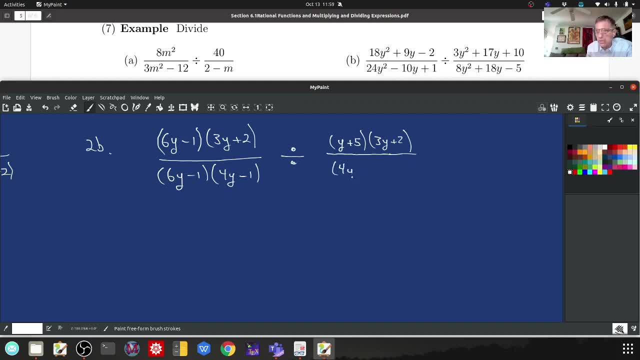 Is 4y minus one Times 2y plus five. But notice, I still have this right here. This is the division sign, So I'm going to change that division sign Into multiplication sign. There I did it, And what do I have to do? 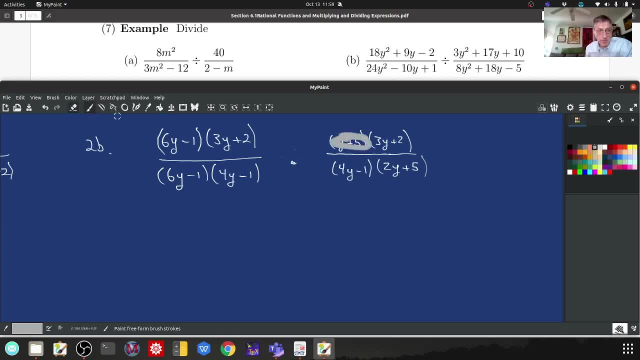 Well, maybe it would help if I had the eraser. I have to flip exactly all of what I just wrote there. The numerator becomes the denominator And the denominator becomes the numerator. That's a big, huge multiplication sign. No ambiguity about that one. 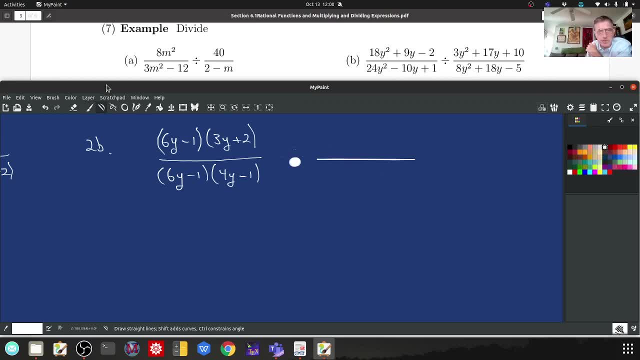 Okay, So that gives me on the top 4y minus one times 2y plus five, And y plus five over 2y, Y plus five, 3y plus two. So now we just everything is factored into linear factors. 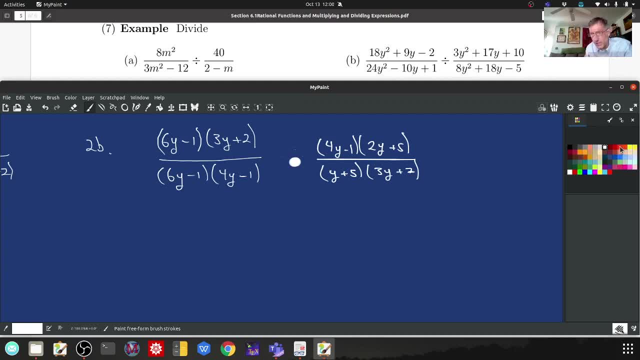 So once you've done all of this, this is probably actually easier. Is there a 6y minus one? Yep, there sure is 3y 3y plus two. Yep, there's a 3y plus two. 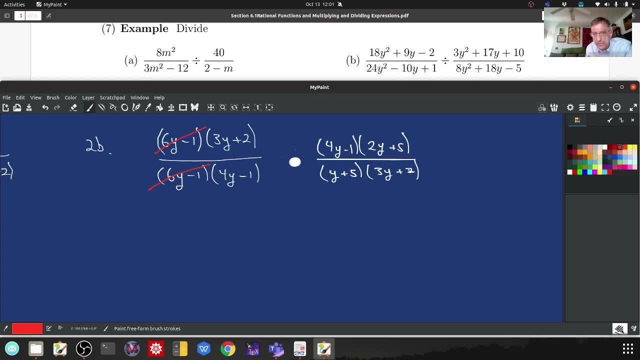 That's supposed to be a plus two. there Doesn't look like it, but I don't know if I just was lazy about writing it. But let me make sure you realize That's all I have to do. That's supposed to be a plus two. 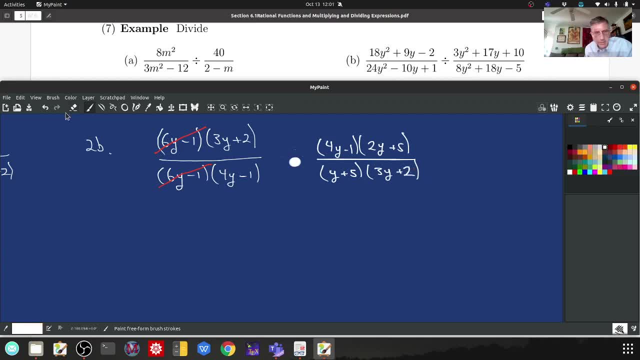 There we go. So there's a 3y plus two And a 3y plus two 4y minus one. All you have to do is look at the numerator: Go factor, factor, factor. 4y minus one. 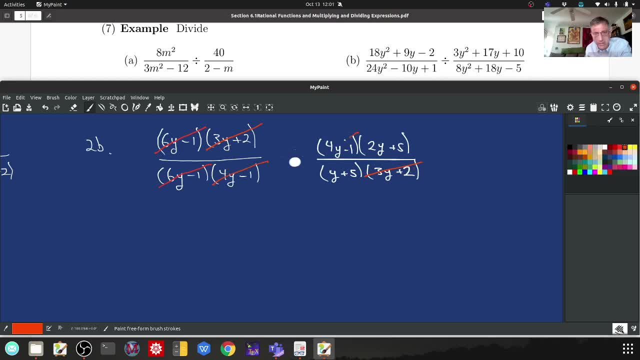 And here's a 4y minus one, And here's a 4y minus two, 2y plus 5 and a y plus 5.. So all of this is equal to 2y plus 5 over y plus 5.. 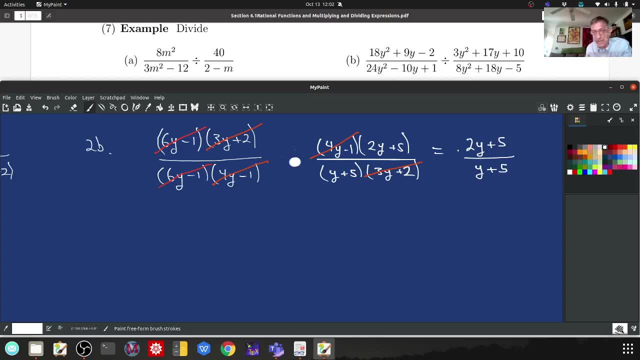 And that's it. These cannot be simplified. You can't do anything to that, Because this is a prime linear binomial: 2y plus 5.. Can't be factored: y plus 5. Can't be factored. 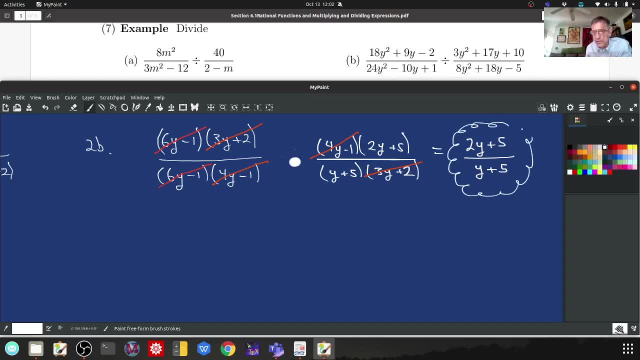 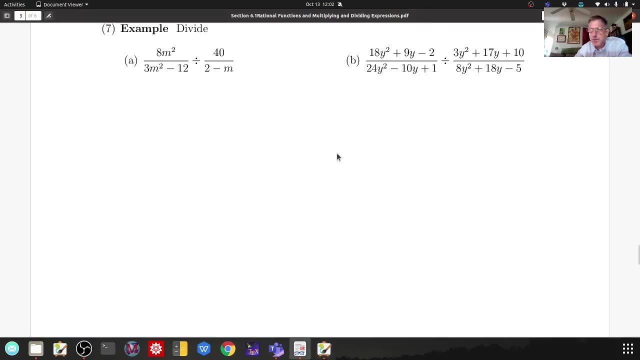 So this is it, You're done. Resist the temptation to cancel the 5s. That's really bad. Do not do that, And I'm going to leave a challenge for you, This one. So let's do this. I can't do this. 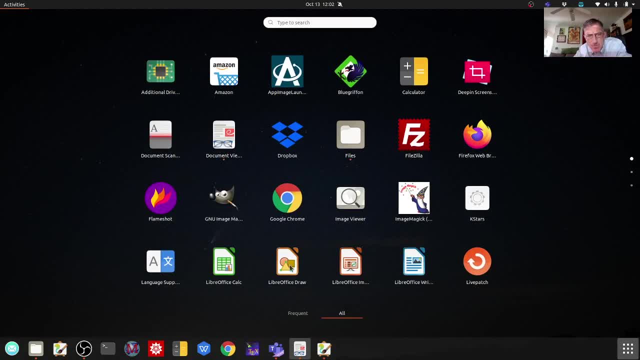 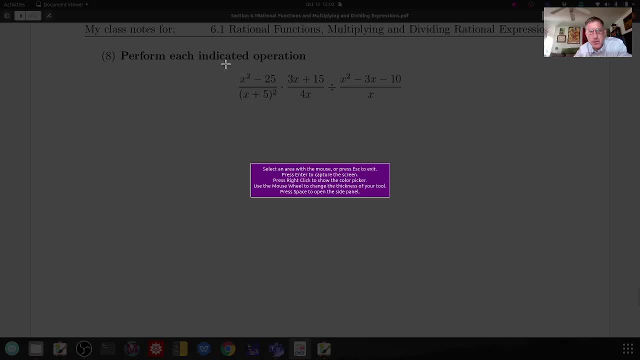 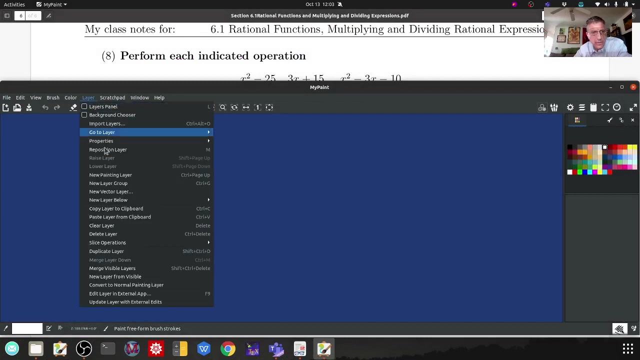 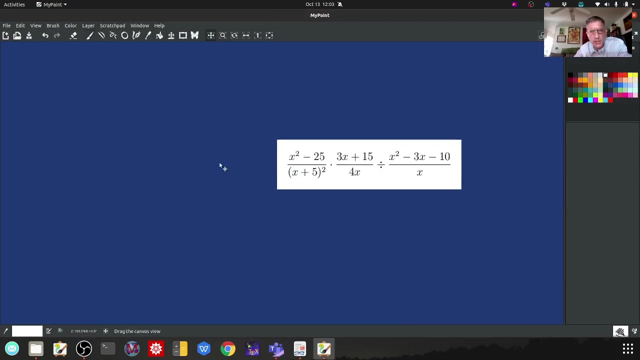 Where is my thing? Flameshot, I'll take a screenshot, Screenshot. So here is the deal: We're going to use PEMDAS. The only thing about this one: I'm going to let you do it on your own. 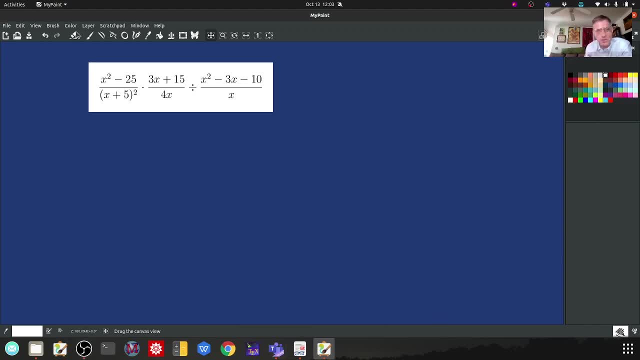 But I'm going to give you a hint And I'm going to give you the answer. So this is PEMDAS, So there are no parentheses, So I can't use that one. There are no exponents. There are no exponents to deal with. 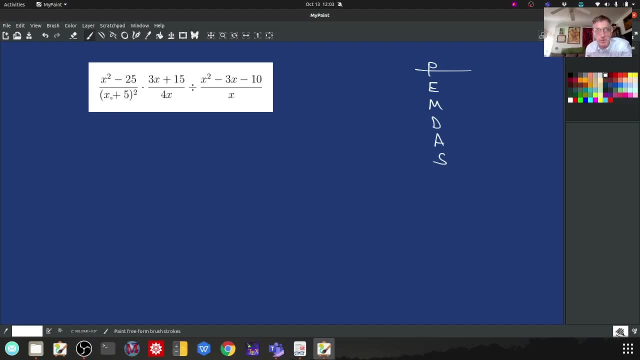 You do not expand x plus 5. You leave everything factored. So then it says If we have multiplication And division, They come next In the order They appear. They appear Going, Going left to right. So all we do is 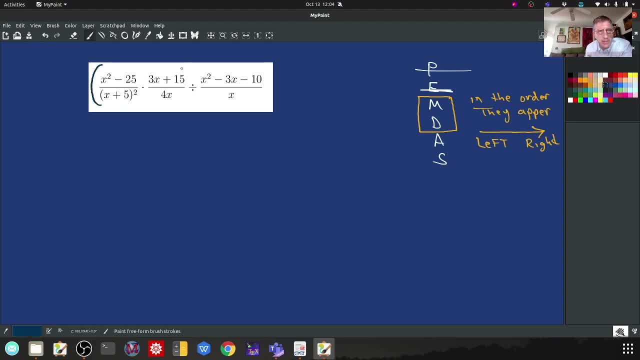 You can put parentheses here And you simplify This first. So that's the order you're going to do. You're going to do: Find out what this expression is And then divide it by this expression. So the end result: Once you do it all. 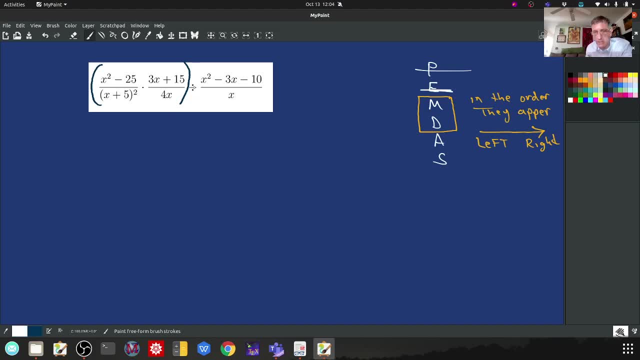 Remember, then This is going to be division, So you're going to have to change this To multiplication And invert this part right here. So the end result, The end answer Is: Are you ready for it? Three Over four: 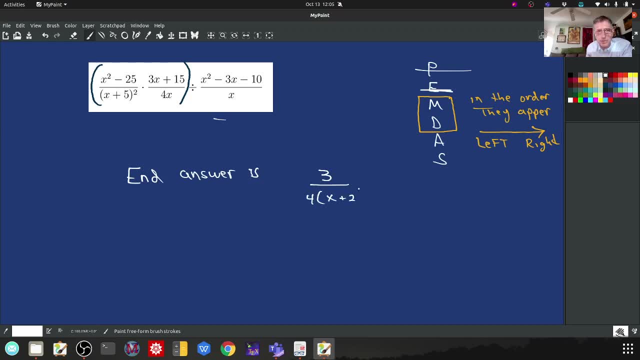 Times x Plus Two X squared minus 25.. That's the difference Of perfect squares: Three x plus five. Factor out of three X squared minus three x minus ten. Just use your regular factorization. There's nothing that can be done with the x term. 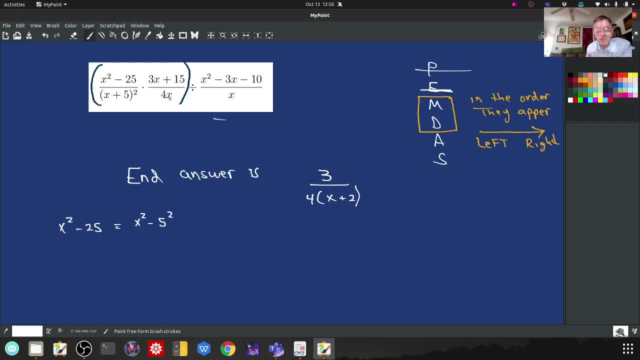 As far as factorizations, Nothing can be done with the four x, It's factorization. Do not expand x plus five To x squared Plus ten, x plus twenty five. Leave it as it is, But just remember That x plus five. 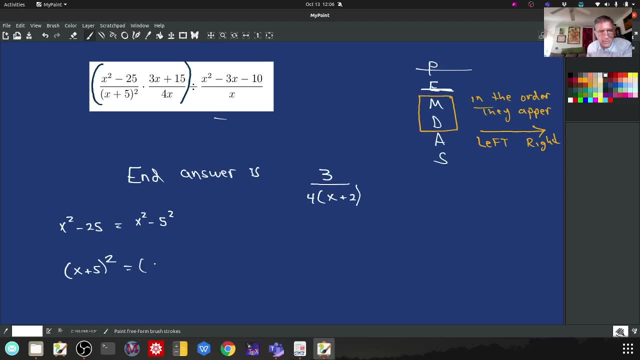 Squared Is equal to x plus five Times x plus five, And this should be your final answer. If you attempted And cannot get it, Just send me an email. Tell me which one it is. It's lecture for 6.1.. 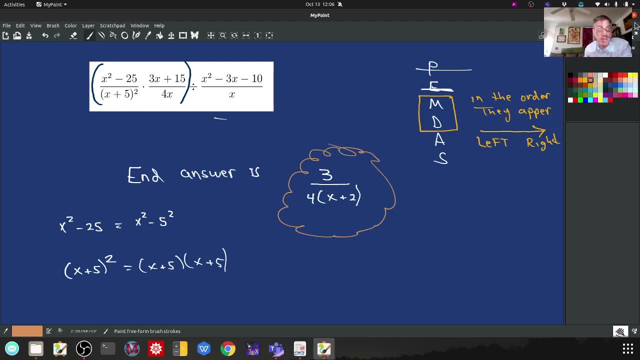 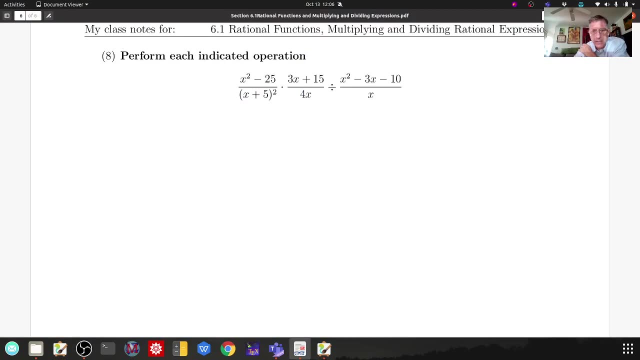 Problem eight And I will work it out Or take a picture of it And send it to you. So let's do this last Problem. It's an applied problem: Cost for pressing compact disc. It's a rational expression For the ICL production company. 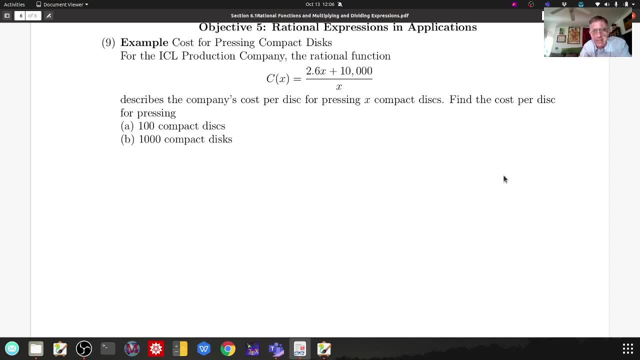 The rational function C of x Is equal to 2.6. x Plus ten thousand over x Describes the company's cost Per disc For pressing x compact discs. Find the cost Per disc For pressing One hundred. 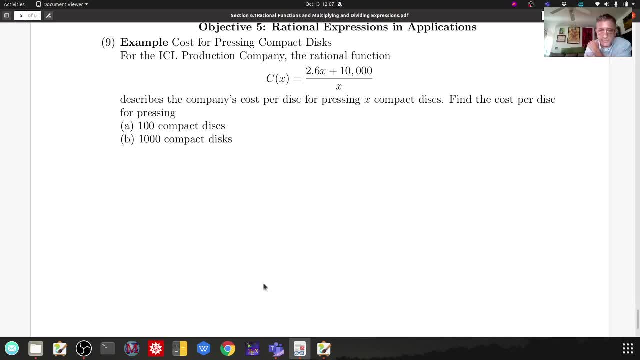 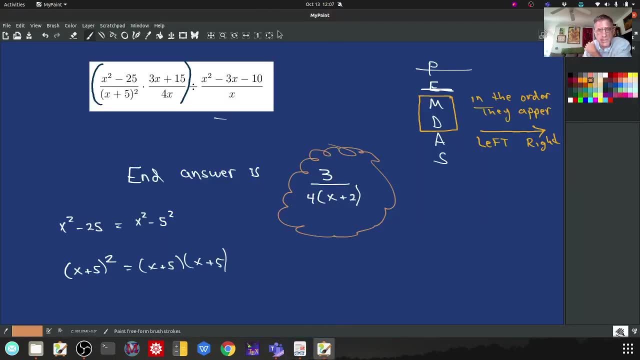 And one thousand. I'm just going to do one of these And then I'll let you do the other These. This is the simple, Simplest of all Applied problems we can have, Because we're literally given A function. 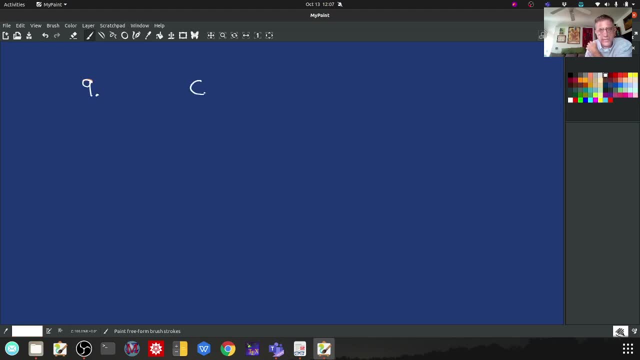 It's a rational function, It's a cost function. C of x Is equal to 2.6.. Times x Plus Ten thousand Divided By x, Provided X Is not equal To zero. And what does our x stand for? 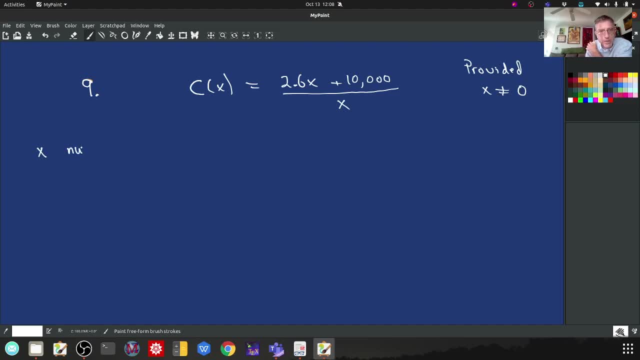 It's X stands for The number Of cds Pressed. You know it's funny. I'm old enough That everything was Final records. And then we went to cassette. No, Then we went to eight track tapes. 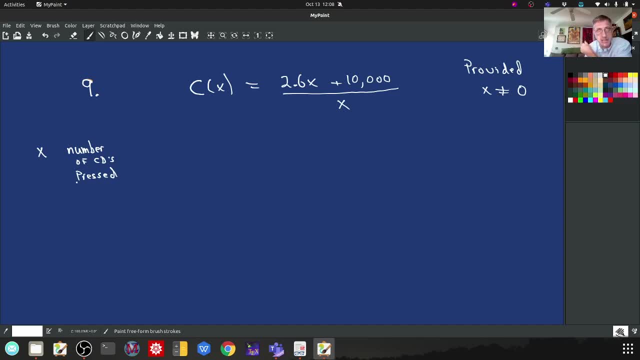 Which was In tapes, Then we went to cassette tapes And then the cd hit And the cd placed, every Replaced everything. And then the next thing you know, Dvds have replaced everything. Then all of our memory Got really small. 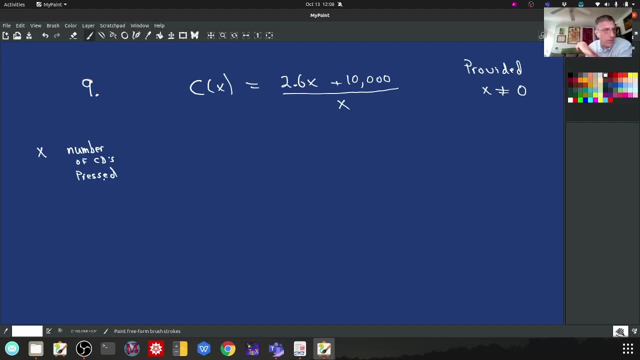 And it all became digital, Or Your thumb drives Or your little Miniature Sd cards. Oh how things have changed. So they want you to find. Part a is literally asking To find The value of c Of 100. 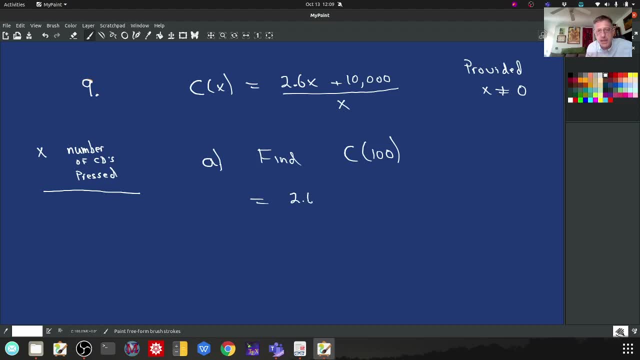 So all we do is we just replace X Times 100 in this case, And we Perform The arithmetic, and there is absolutely no reason That you need to use a calculator for this. And for those of you who are really calculator dependent, 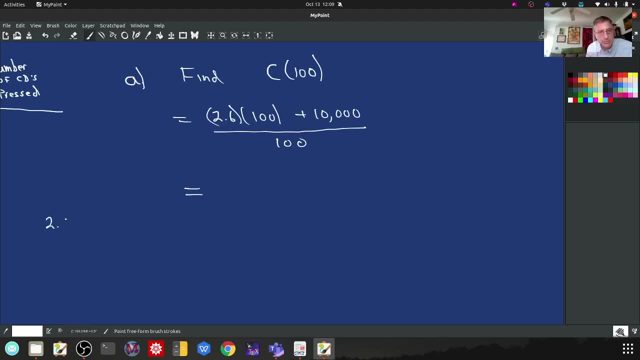 So 2.6 times 10. Is equal to 26.. You just move the decimal over. So 2.6. Times 100. Is 260.. So you just multiply, You just move when you're multiplying by. 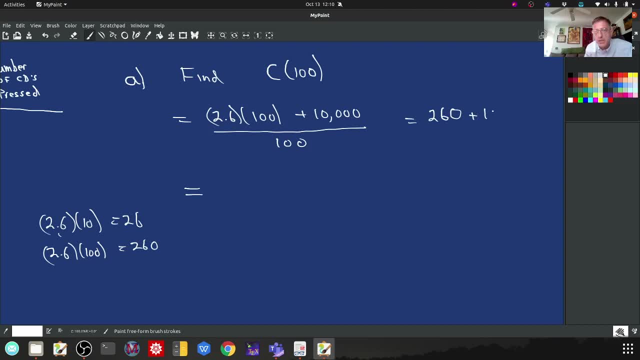 The power of 10.. I use it's really, especially if decimals are involved. You just move the decimal, So this is 10,000.. 260. Divided by 100.. So here the world on trick. I have a zero up here, is zero up here. 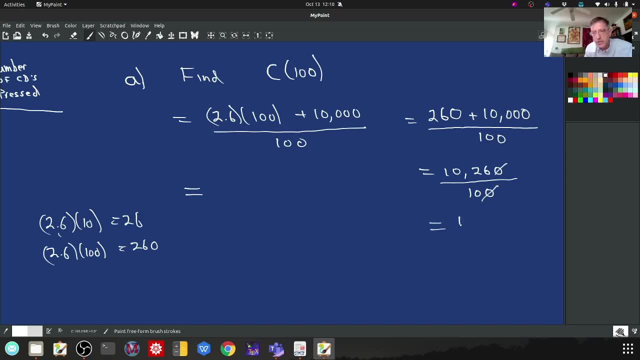 So I can cancel out one zero, So that's 1000.. 26. Divided by 10. That means I just take 1000 and 26. And move the decimal over, So it's 102 dollars, And